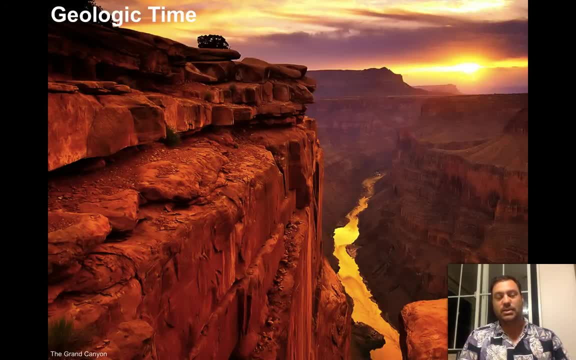 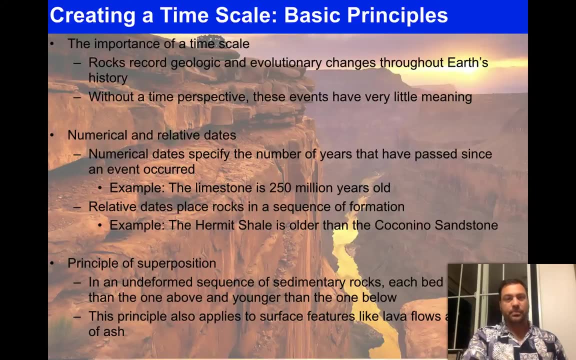 creating the canyon that then exposes that rock. for us, It takes a tremendous amount of time to be able to do this. How do we know? You're going to see how we know that now. All right, so we need to establish some basic principles as we go forward. right, One of the things that we need to come up with is how we measure this time, And usually we think of it in terms of minutes and seconds and hours, That's, in our day-to-day human life scales. 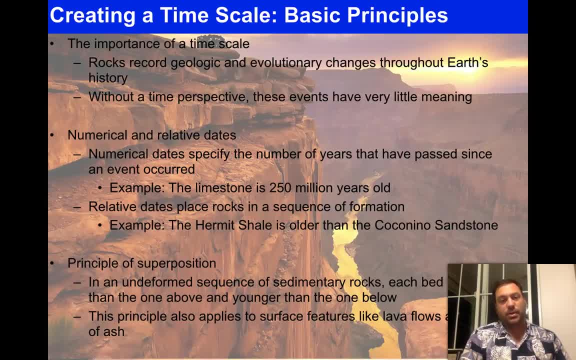 But in the geologic time scale, we're dealing with a lot longer periods of time. We're dealing with periods of time that could be millions of years, right, Billions of years in some cases. So if that's the case, we need something a little different. So we need a time scale. 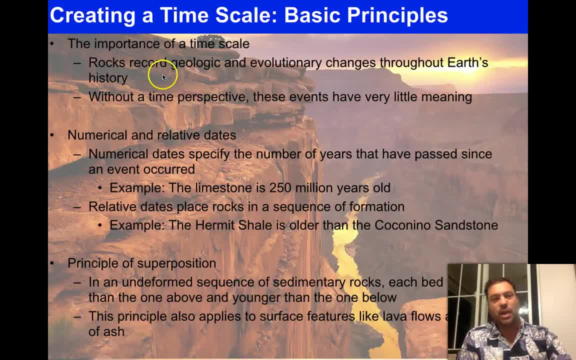 Well, rocks. so let's talk about the importance of a time scale. Rocks record geologic and evolutionary changes throughout Earth's history, But out of time perspective, these events have very little meaning, right? So if it happened 6,000 years ago or if it happened 6 million years ago, we need to know the difference. 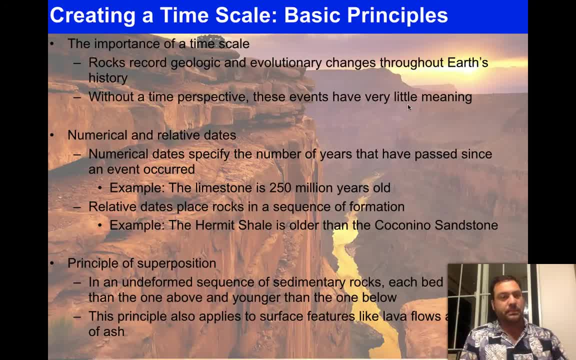 Otherwise we could really get messed up in our conclusions. So there's two ways that we could do this right. We can state things in numerical and relative dates. So numerical dates specify the number of years that have passed since an event happened. It's an actual number, right. 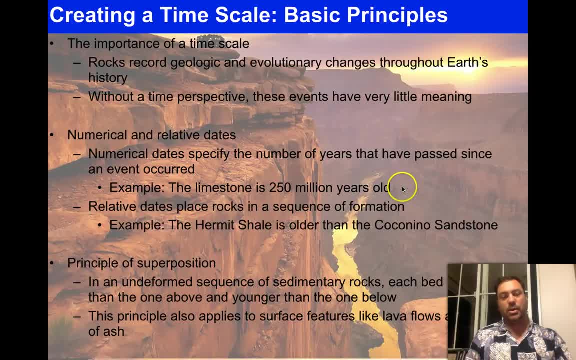 The limestone is 250 million years old. That's an actual number that we can apply to it. By contrast, we have relative dates right. Relative dates place rocks in a sequence of formation, So the Hermit's Shale is older than the Coconino. 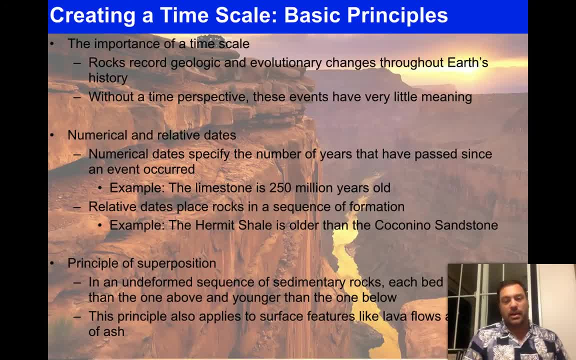 We do this all the time, right? It's one thing to say that if you're, say, 20 years old and your little brother is 15 years old, those are absolute dates, right? There's a five-year difference between the two of you. 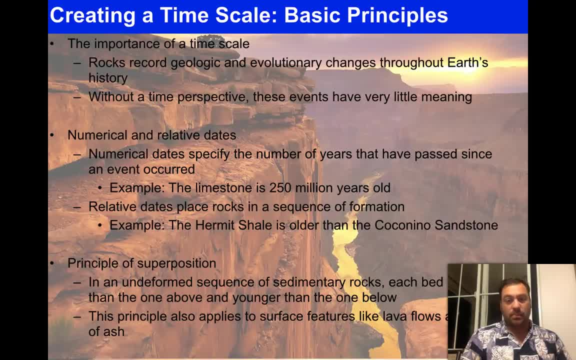 But if you just say he's my little brother or my younger brother, then we don't really know what the age difference is between you. We can glean that if we look at you. maybe we can get some idea, but we really don't know how old or that age gap is right. 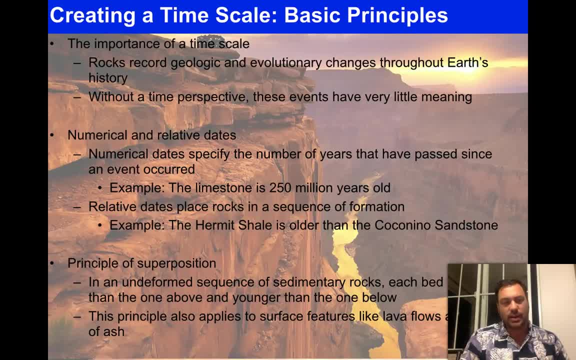 Unless we have that information All right. so you get the idea right: Relative dates versus numerical dates or absolute dates. Of course, one of the most important principles that we need to start off with is the principle of superposition. It's almost too commonsensical to really go over, but it is in fact important to talk about, because everything else kind of built off of this. 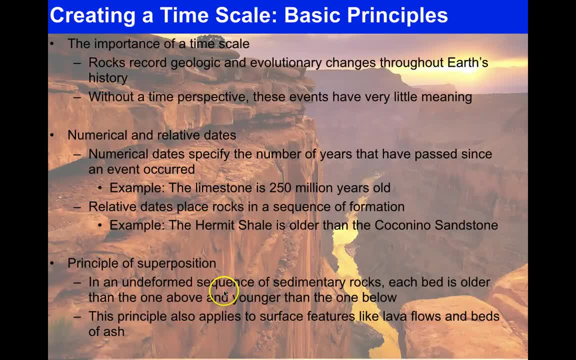 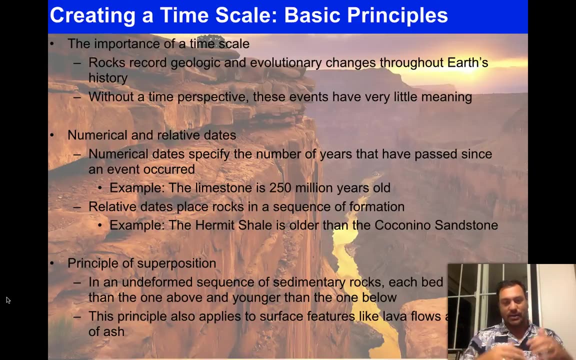 So, in an undeformed sequence, you know a series of layers of sedimentary rocks. each bed, each rock layer is older than the one above And younger than the one below. So, provided that there's been no problems going on during the deposition of rocks, the oldest one's going to be the oldest, or the bottom one's going to be the oldest and the top one's going to be the youngest. 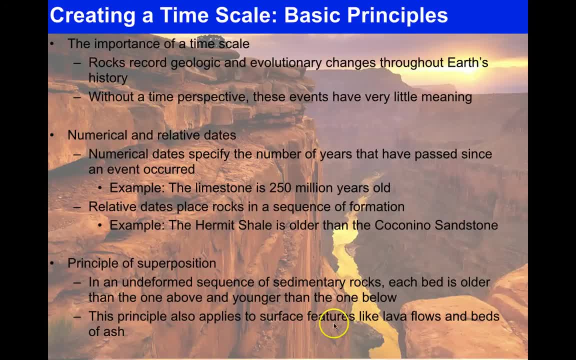 That's the principle. And this principle also applies to surface features like lava flows and beds of ash. So you're not going to get a lava flow that's going to creep underneath other lava flows. generally speaking, They're going to pile on top of one another, so that the youngest one is on top and the oldest one is on the bottom. 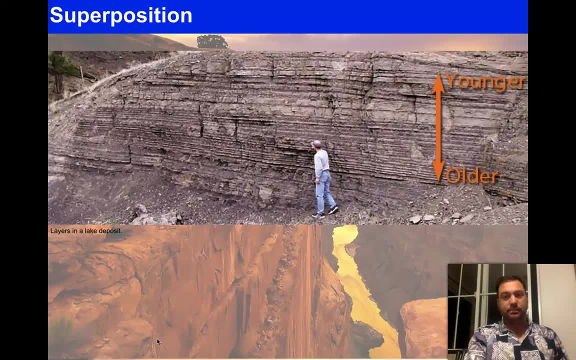 Same thing with the bottom, Same thing with the bottom. And so here we see this kind of illustrated in this diagram here. Here we see this scientist looking at lake deposits. The obvious thing that we get out of this is the lake deposits do not appear to be deformed in any way. 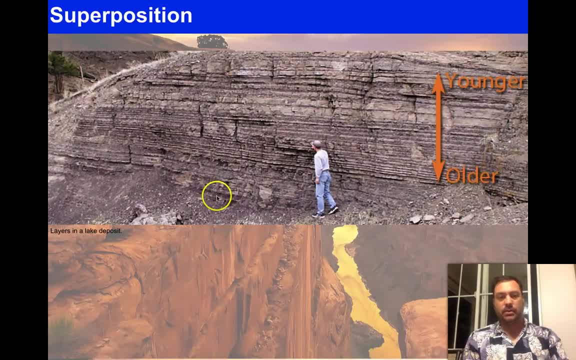 They're nice and flat. And so we can apply the you know principle of superposition and surmise that the older is going to be on the bottom and the younger is going to be on the bottom. And so we can apply the you know principle of superposition and surmise that the older is going to be on the bottom and the younger is going to be on the bottom. 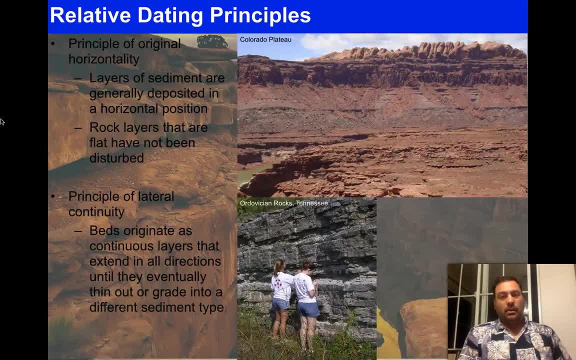 That's the idea. Okay, Now there's some other principles. we need to bring up The principle of original horizontality. So layers of sediment are generally deposited in a horizontal position. That means flat line. Okay, Rock layers that have- I'm sorry, rock layers that are flat- have not been disturbed. 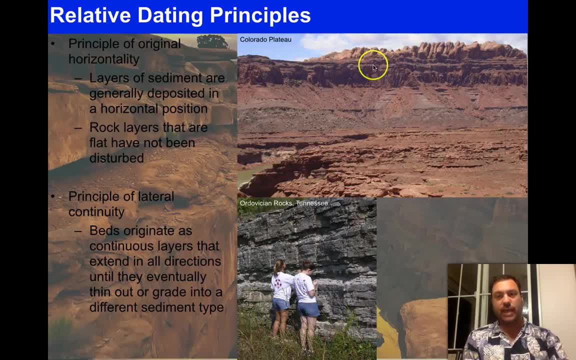 Right. So here we see on the Colorado Plateau. we see these rock layers: nice and flat, flat, flat, everywhere throughout here. Here we see in these Ordovician rocks the same thing: Nice, flat layers, Right, Not deformed. 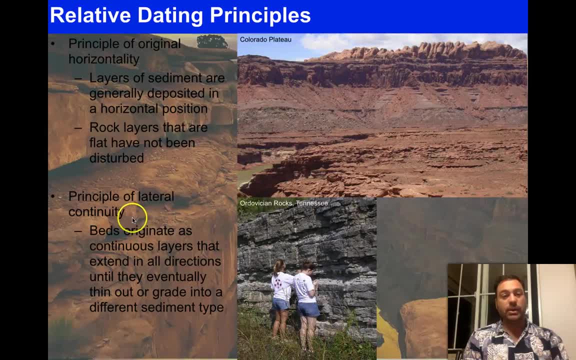 Not disturbed The principle of lateral continuity. Beds originate as continuous layers that extend in all directions until they eventually thin or grade out in a different sediment type. We can see that here. Right Rocks that are on one side of this little gully are probably the same rocks that are on this side of the gully. 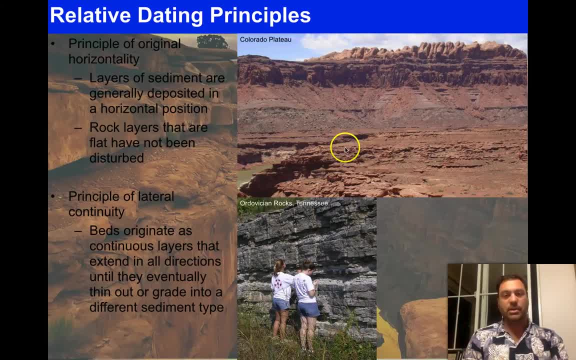 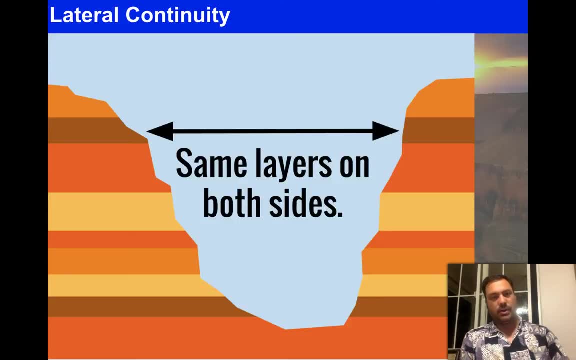 It just extends across Right They probably they were continuous at one point. There wasn't originally this gap here And we can see this demonstrated here. This lateral continuity is that originally there was a rock layer that extended across the valley here. 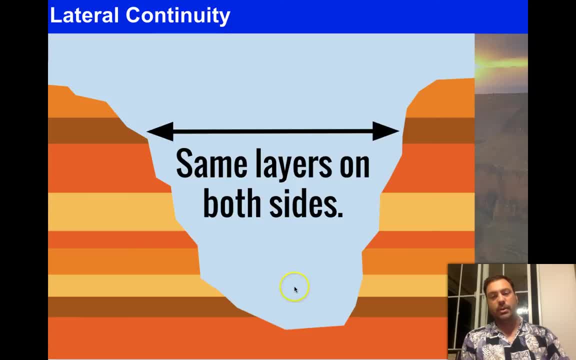 And when this valley building event- whether it be glaciers or rivers- carved this valley out, it left it on one side, But at one point it was continuous. That's the principle that you need to get in mind And, as a matter of fact, down here it's still relatively continuous, except for this part. up here on the top. 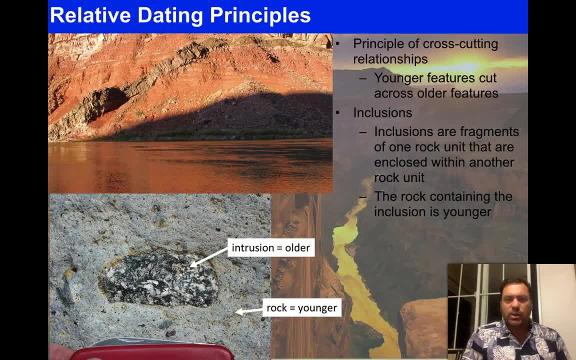 All right. another really cool principle- and these are really really neat in geology to find- are cross-cutting relationships. This is where something cuts across: an older feature, something that is young. So here we see a bunch of layers. 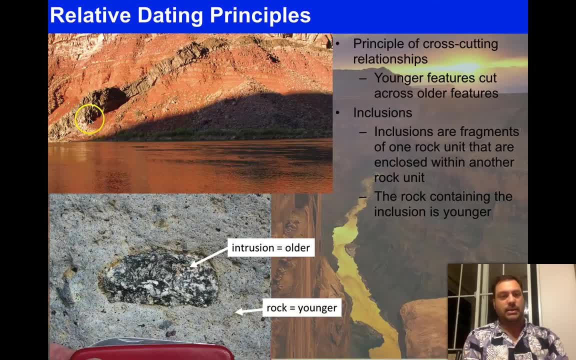 You can see the layers here, And cutting across it is a dike, And notice that the dike is not going in the rock layers, It's cutting across, And so the question you have to ask yourself then is: what is older? Is the dike older? 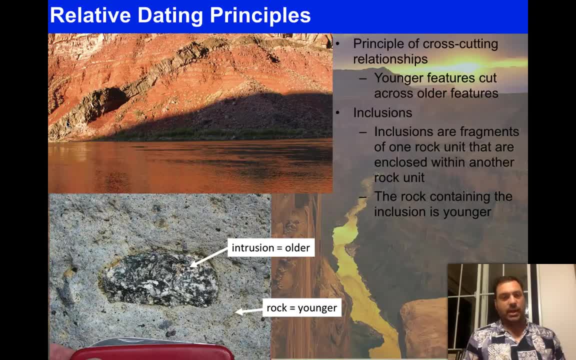 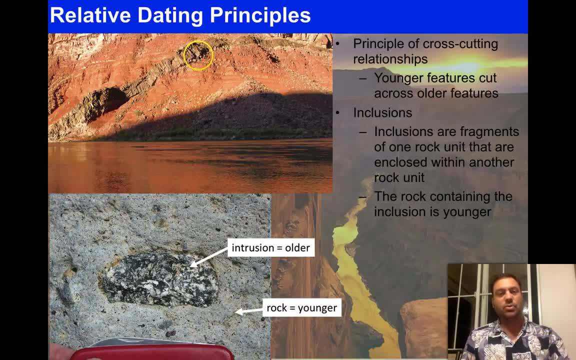 It's. you are intruding something that is cross-cutting, something that is flat. This is undeformed and probably came in this way. This came in much later. Okay, Inclusions. Inclusions are fragments of one rock unit that are enclosed within another rock unit. 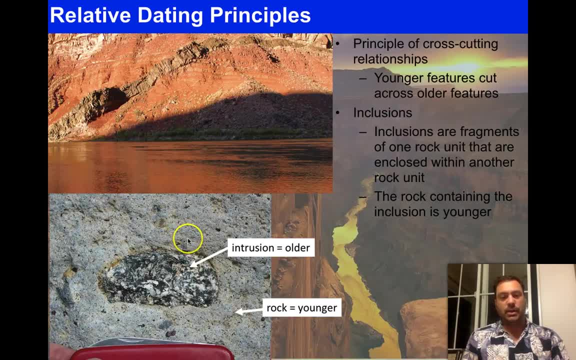 So here we see- in this case this is an igneous rock. We see a rock right, But the intrusion or the rock that's stuck inside of it is actually younger, And this is pretty common- that we find bits of rock stuck in other rocks. 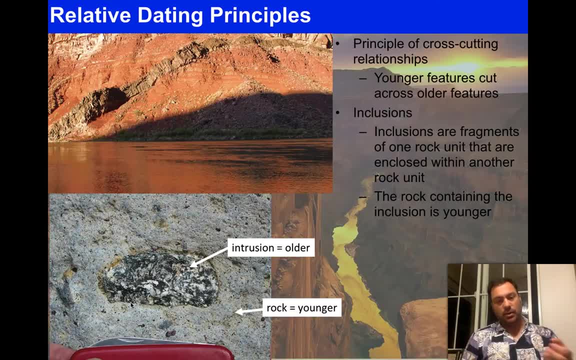 As a matter of fact, that's what sandstone does: right Sandstones and conglomerates and breaches. they're little pieces of rock that are older that are now in a much younger rock, say a sandstone, And in this case we see a bigger clasp, a big piece of rock that's stuck in another one. 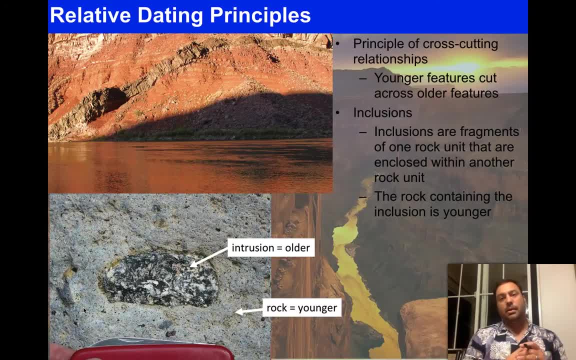 And this happens where, say, a brick, A volcano is erupting and during the process of erupting it grabs, or the lava is moving up, it grabs off a piece of the country- rock, or the side wall rock- and takes it up with it. 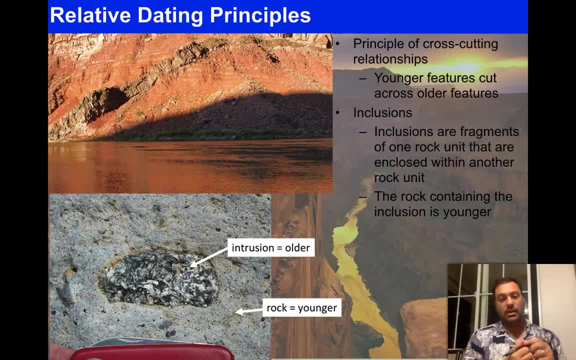 into the volcanic eruption And then we find it up here on the surface. okay, That's kind of a normal way. you get an intrusion. So in this case, the rock containing the inclusion is younger, So here's younger. This, of course, has to be older, right? 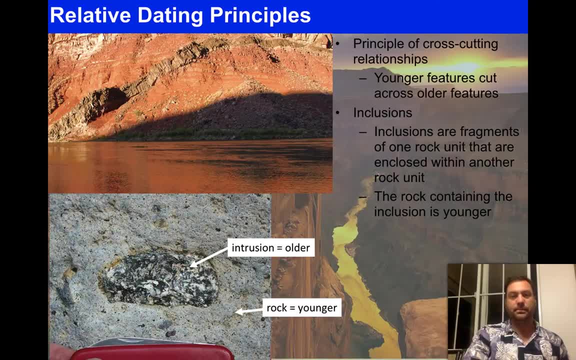 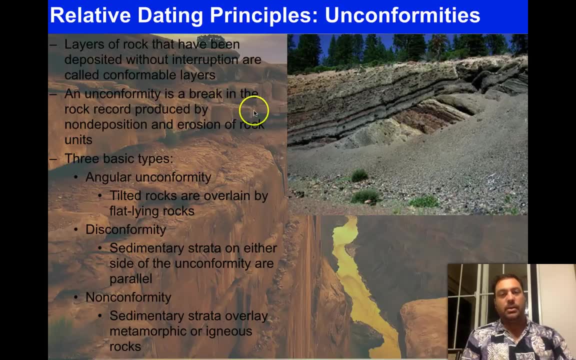 This has to exist before it can be a part of this rock. That's the idea, All right. Another. these are really really neat, And here in Hawaii, where I'm recording right now, we see a lot of these types of things. 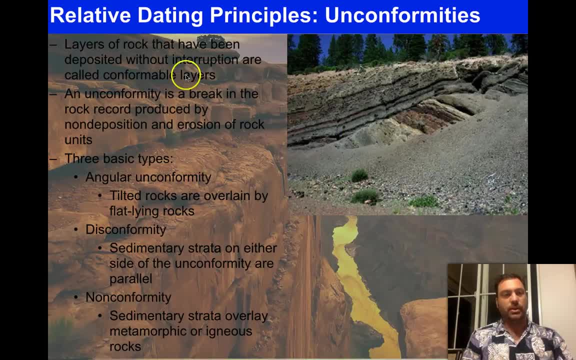 these features over here. These are called angular unconformities. We're going to come to these here in a moment. So layers of rock that have been deposited without interruption are called conformable layers. In other words, where things just continuously happen and change, it's all conformable right. 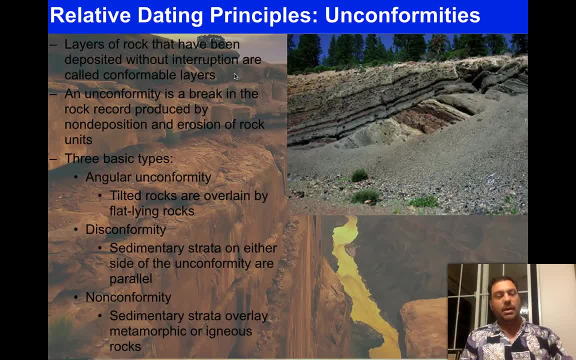 There's. it's a continuous recording of time, But an unconformity is a break In the rock record produced by non deposition and erosion of rock units. In other words, a period of time where or location where, for whatever reason, that deposition stops right. 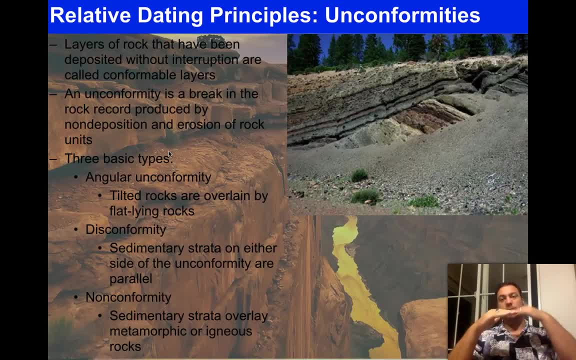 The layers just stop forming. They might take a break for a while and then form again, But it's basically a period in geologic history of lost time, right where we don't see that record anymore And sometimes maybe you might have layers being deposited. 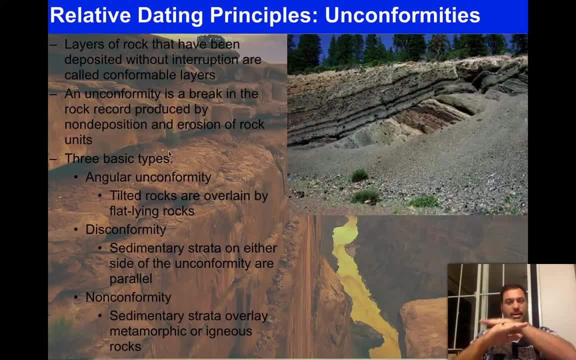 You get some type of tectonic event like a fold that gets all eroded off, So it destroys everything off the top, and then it starts to pile more stuff on top of it again. That's one way you get an unconformity. 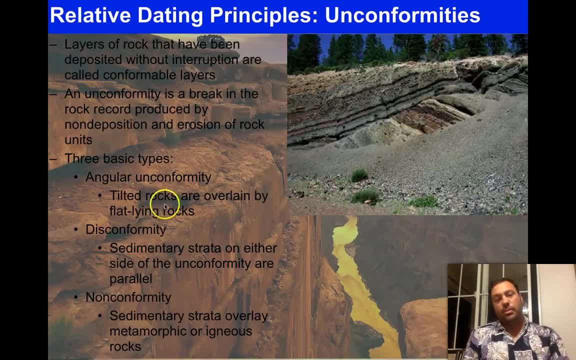 So there are three basic types. So an angular unconformity is just tilted rocks that are overlaid by flat line. So that's what this is here. So here we see some nice angular or rocks that are at an angle. right here, Some erosion has happened along its edge and since then these new layers have been, or these new layers have been. 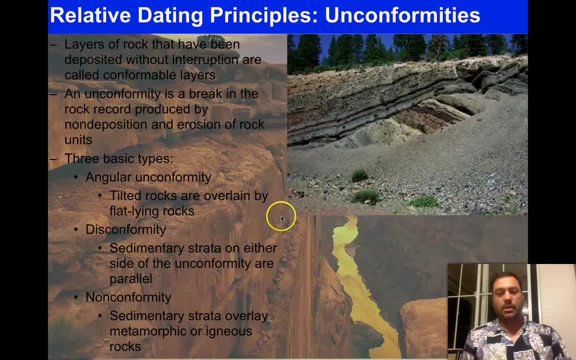 deposited across the top and those have been tilted. even They're in that outcrop. Okay, so other than an angular unconformity, we can go to a disconformity. A disconformity is simply sedimentary strata on either side of an unconformity. 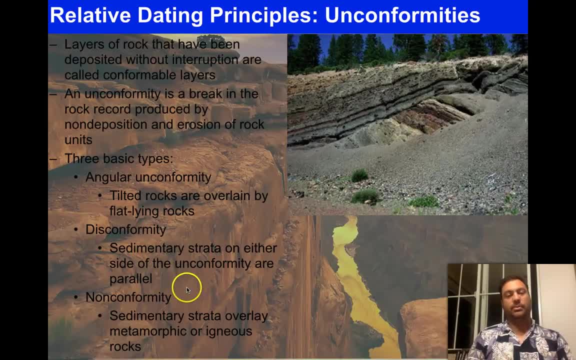 You should say in an unconformity, and they're parallel. right, They're going to be parallel. In other words, you have a layer that's put down, There's a period of missing time, and then all of a sudden more comes in again, right? 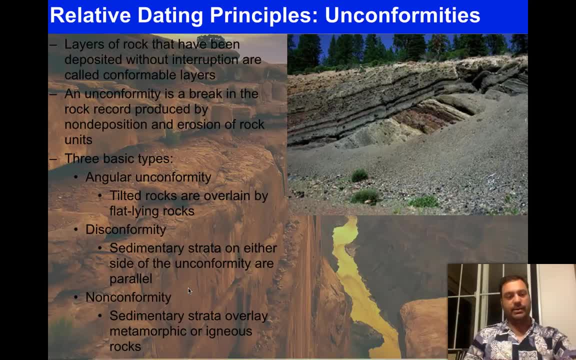 So there's just a period of missing time and everything's parallel, nice and flat. A nonconformity. is sedimentary strata overlaying metamorphic or igneous rocks, right? So in other words, when the igneous rock is made, 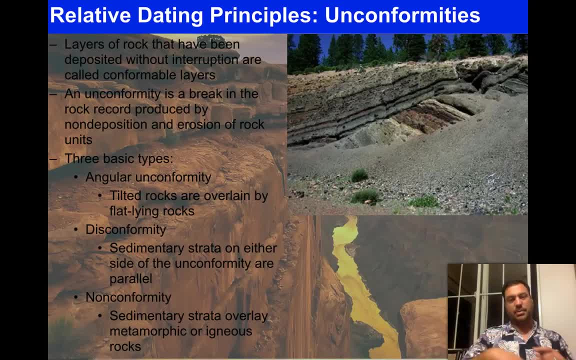 it's not recording fossils or anything like that. As a matter of fact, igneous rocks destroy fossils and then, for whatever reason, it might, get beveled off into a nice flat surface and you get sedimentary layers put on top of it. That's when you get the real recording of real time, almost like a tape recorder. 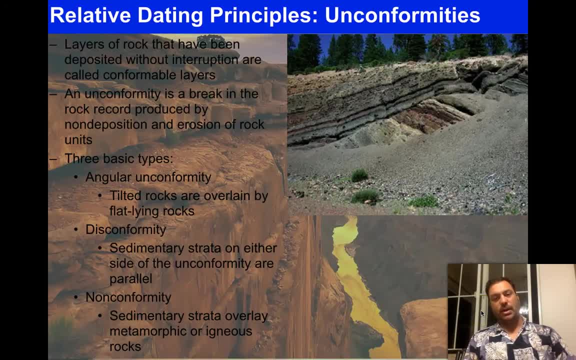 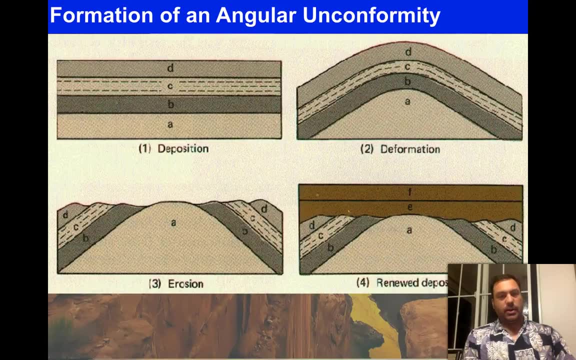 The difference between that igneous rock and that sedimentary rock. it's called a nonconformity. So here's an example of how you would create an angular nonconformity. right, You get deposition, deformation, you get erosion, where you basically chomp off the top of these rock layers, and then you renew the deposition. 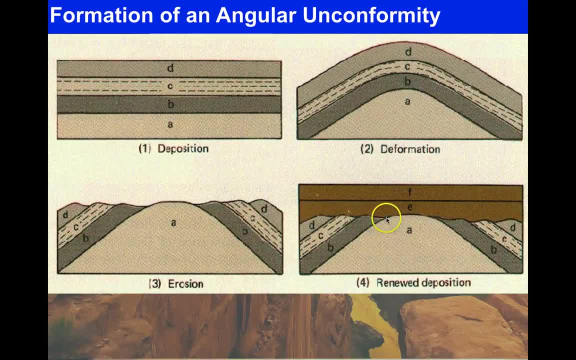 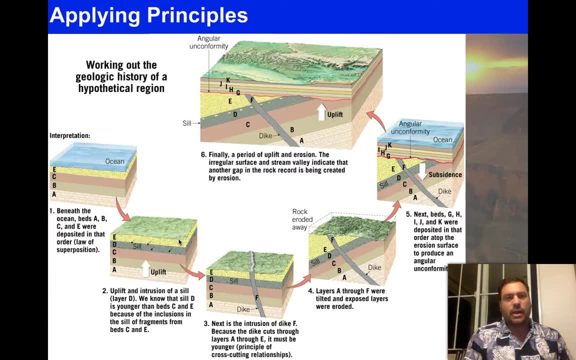 You get these angles over here, So you get an angular relationship right in here, And there's different ways that you can work out a hypothetical region, Not necessarily Knowing this information right. So here we have: maybe we go out and map it, or we get seismic data and we see the land that looks like this: 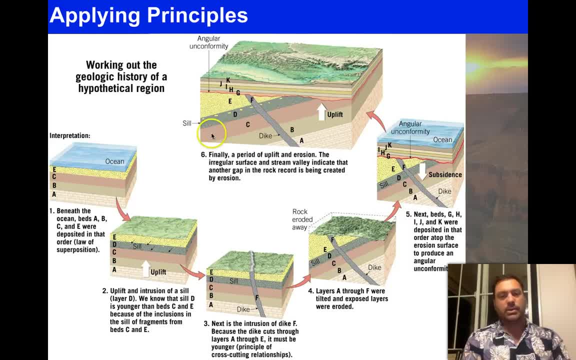 And what we can do is we can work back. The way this works here is actually working towards creating this, But you can work back also, right, And figure out what happened by using the crosscutting relationships, and we can figure out something. 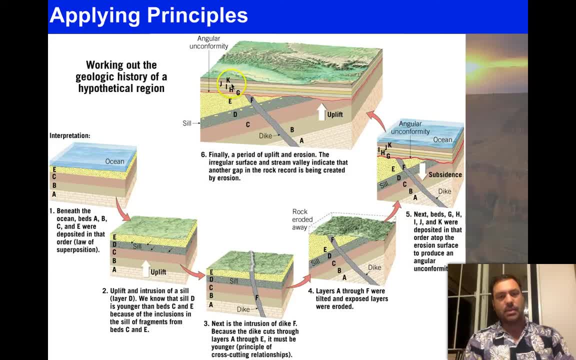 For example, we know that K has to be much, much younger than A, And we know that the dike had to be younger than A, And we know that the dike had to be younger than both A, B, C, D and E. 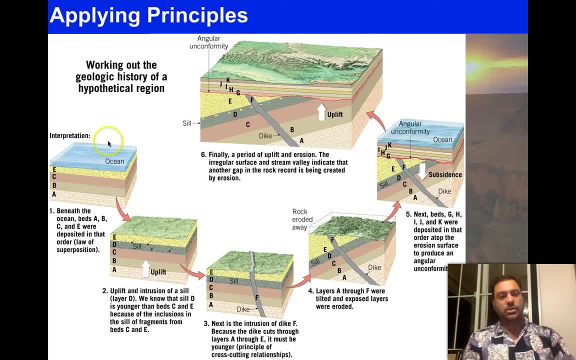 Okay, There's a lot of different things that we can put together, And so there's an interpretation. right, We got some layers that were put in, maybe in an oceanic environment, So this would be the law of superposition. From there, we can intrude a sill. 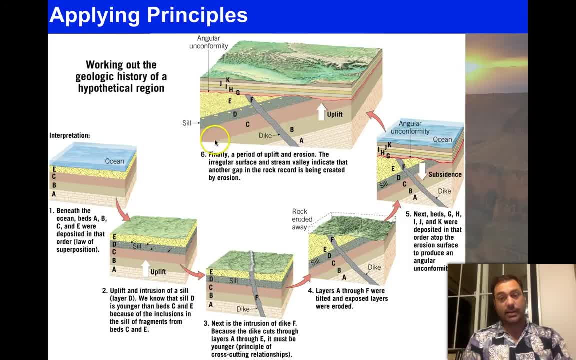 So this would be the sill right here. The cool thing about a sill is that we can date that. We'll talk about how we can do that later on. We know that sill D is younger than beds C and E Because of the inclusions of the sill of fragments from beds C and E. 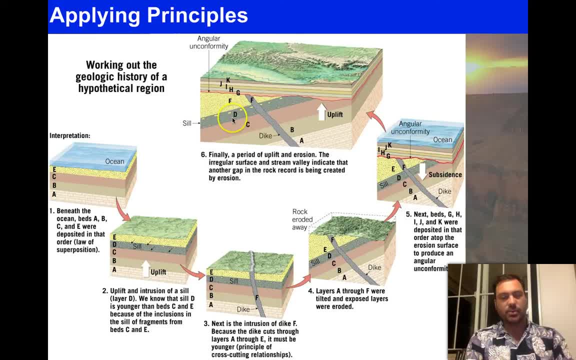 So in other words, we have a bit of E in D. That's what we see there. That's the law of inclusions, right? So next is the intrusion of dike F. So we see another dike come in here. 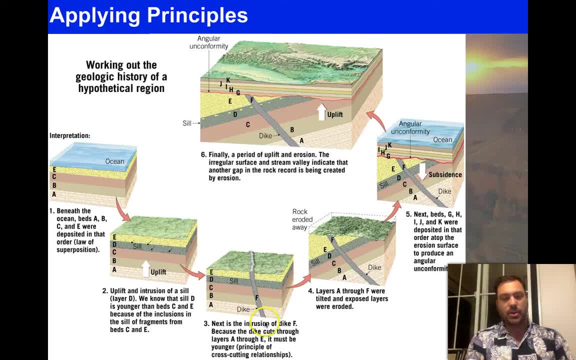 So this is what they believe the landscape will look at sometime, And we know that because it cuts across everything else, Right? And then at some point, this had to be eroded and tilted, Right? So probably, well, of course, the tilting had to probably happen at the same time as the erosion. 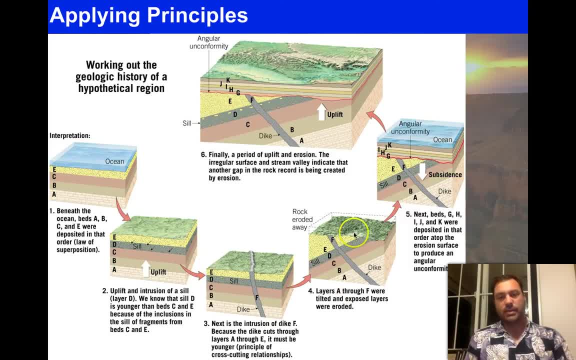 So this gets tilted and eroded, This all gets beveled off. It's nice and flat, And then all of a sudden we get new layers being deposited again. Maybe the ocean comes back. That's what the interpretation they have here. We get G, H, I, J, K- all being deposited. 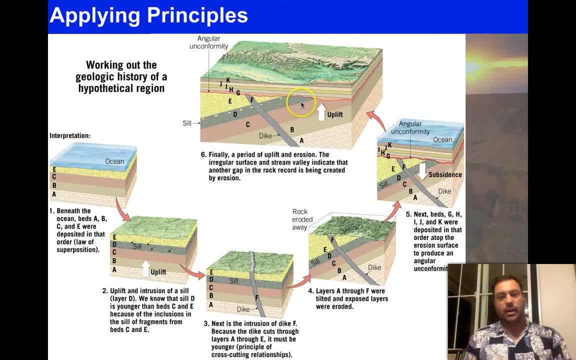 And we wind up with this kind of landscape eventually that we are trying to now interpret Right, So this would be a hypothetical region. This is a real location. So anyway, you get the idea. Take some time, Maybe pause this slide and see if you can work through it yourself. 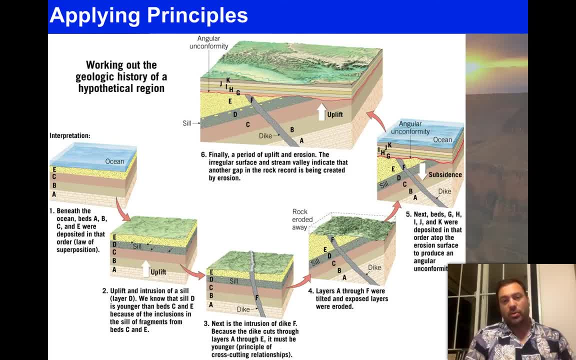 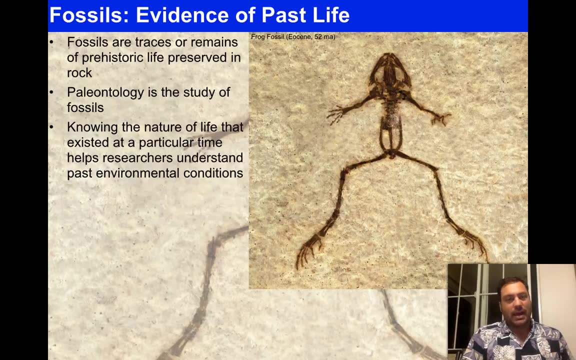 These things are nice little puzzles that you can work through And they're pretty normal homework assignments in a lot of geology classes to work out the geologic history using these laws that I've been covering. Another really neat thing to know about the geologic past is the evidence of past life. 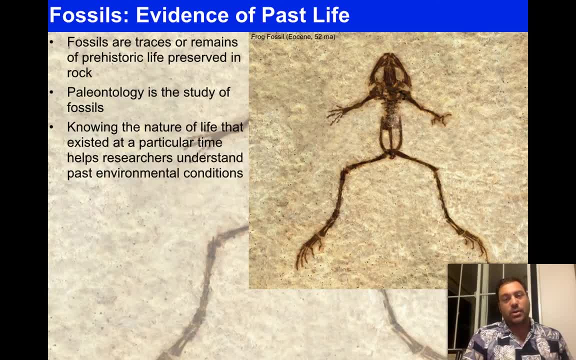 The evidence of past life is usually within the rocks, And if we know something about the evidence of the past life, we can use it to date rocks, So fossils, are traces or remains of prehistoric life preserved in rocks. So here's, for example, a fossil. 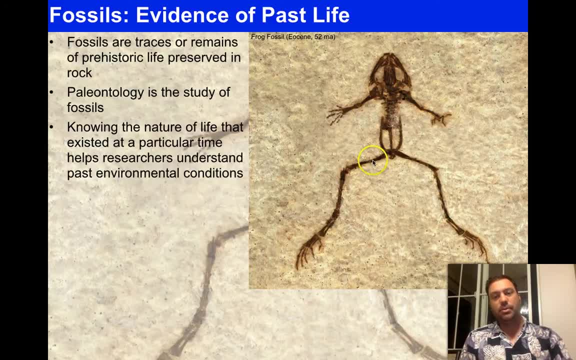 This is a fossil frog. It's 52 million years old And you can tell pretty quickly it's a frog. It looks very similar to what we see today. There are differences. We're not going to get into the differences here, But you know, this is a frog. 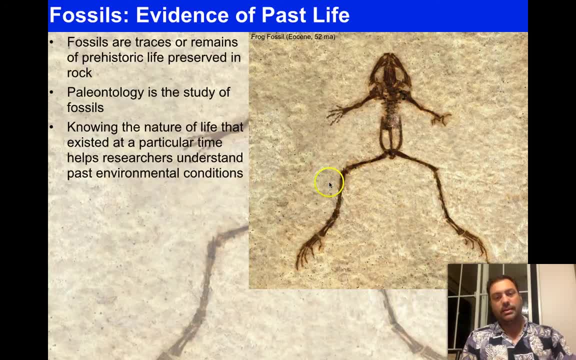 It's 52 million years old And this is kind of the science- Some people would say the art. But the science of going through and studying these fossils and interpreting what these creatures look like and how they lived is a study of paleontology. 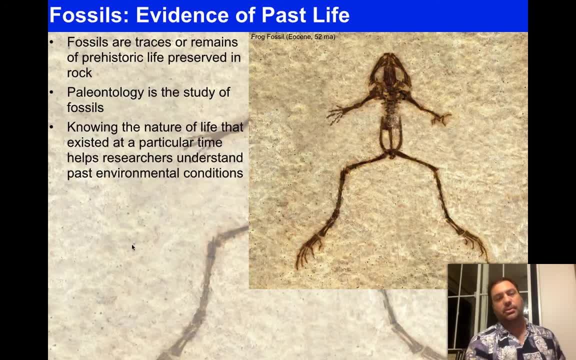 So knowing the nature of life that existed at a particular time helps researchers understand past environmental conditions. Obviously, wherever this creature lived- it's a frog, It's an amphibian- It had to live near water. That gives us clues and insights as to what was going on in that environment that created this fossil. 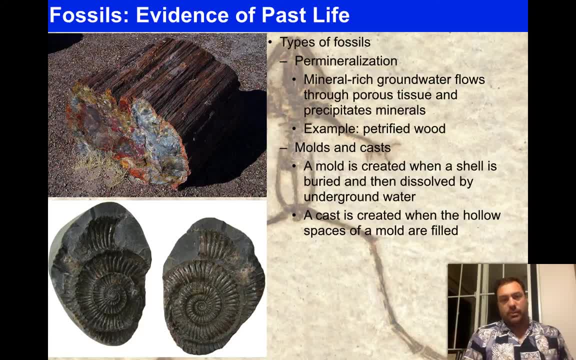 There's different ways that we can fossilize material. We can basically go and make a petrified material here. This is a petrified wood. It's called permineralization. Mineral-rich groundwater flows through porous tissue and precipitates minerals. 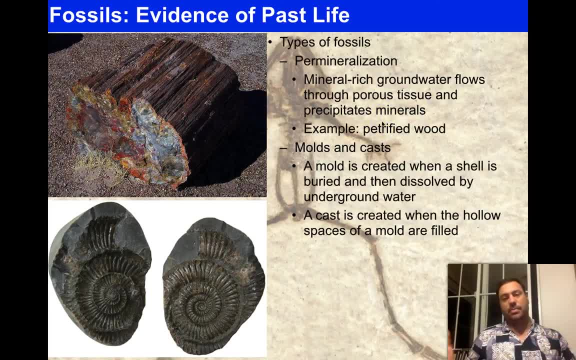 So you get petrified wood, For example. it might get covered by an ash. There's a bunch of minerals that gets deposited in the water- Usually it's quartz or something similar to this- And it winds up being precipitated into the tissue and it replaces it. 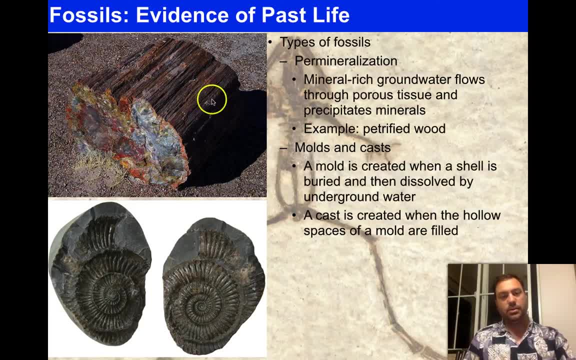 This is actually. even though it looks like wood, there's almost no wood here. This is actually a fossil that has taken the place of the original tree, But you can see that we've got the structures. In some cases we can even get the cells. 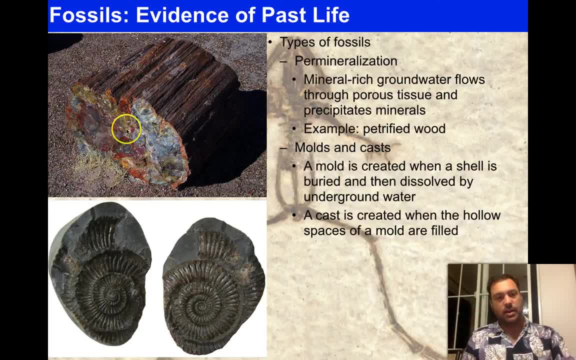 A little bit of information about the cells by looking at these things. Really really neat. Mold and cast Mold is created when a shell is buried in mud. A shell is buried and then dissolved by underground water, So you bury it into the ground and basically the thing disappears. 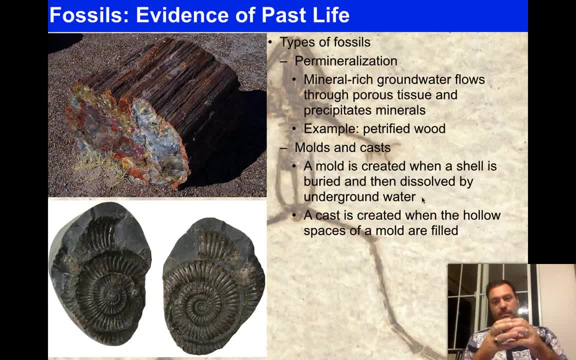 But the hole that is left is the mold right And you can have other things precipitate inside there. You can have quartz, You can have calcium carbonate. All kinds of different things form and replace what was inside that hole And that's called a mold. 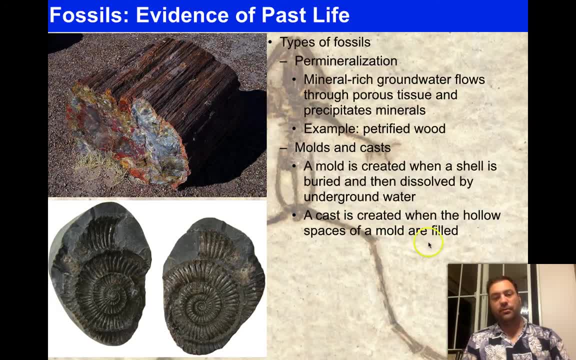 So a cast is created when the hollow spaces of a mold are filled Right. So here we see a mold right here, And here we see a cast where it's filling it in. This is really, really cool. This is actually busted off. 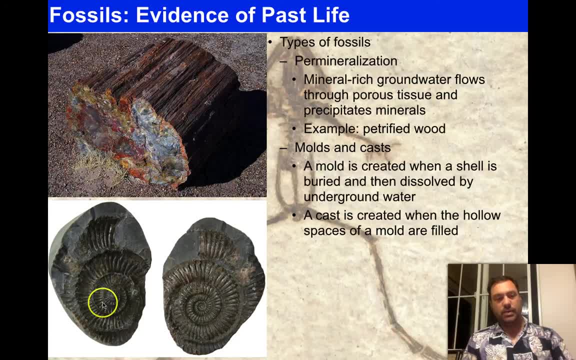 But the original fossil is gone. This is the imprint that it left, This is the mold that it left into the rock, And then the other side basically took on that shape And we can study this creature's features, even though the creature itself is not present. 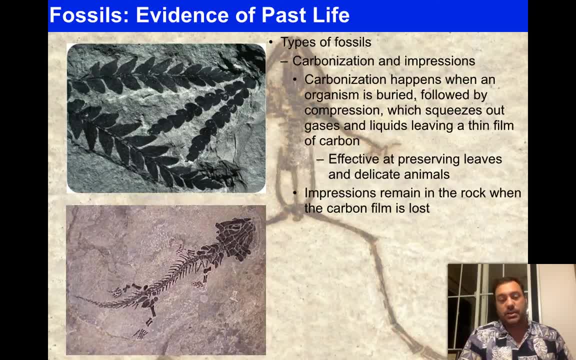 There's carbonization and impressions. This is probably the best way that we know about ancient plants and certain smaller life. So carbonization happens when an organism is buried right, Followed by compression, which squeezes out gases and liquids, leaving a thin film of carbon. 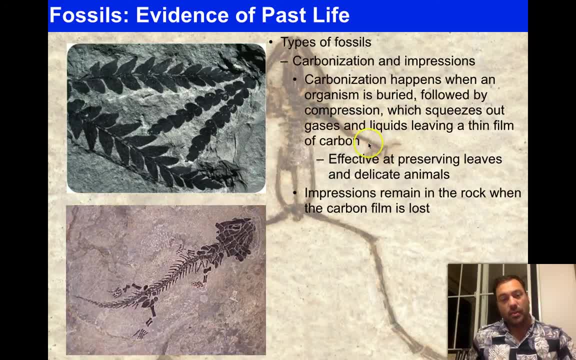 Basically the same processes that make coal, Except for the fact that instead of making coal it goes to a process where it preserves nicely the leaves, And we can see that In fact in coal we frequently do find carbon Carbonization and impressions of leaves in the coal deposits. 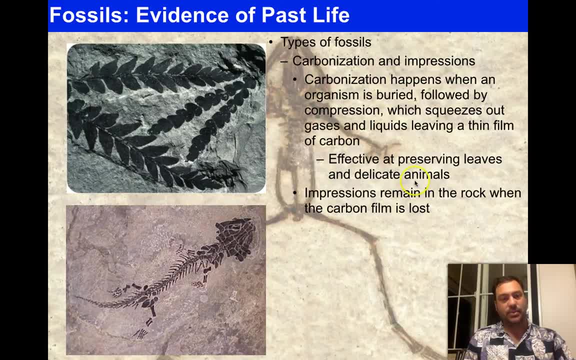 So it's effective at preserving leaves and delicate animals. So we also get some information on the chemistry of the carbon that tells us information about those things, And there's a lot of interesting technology that is looking at the carbon molecules and their arrangements to figure out information about these fossils. 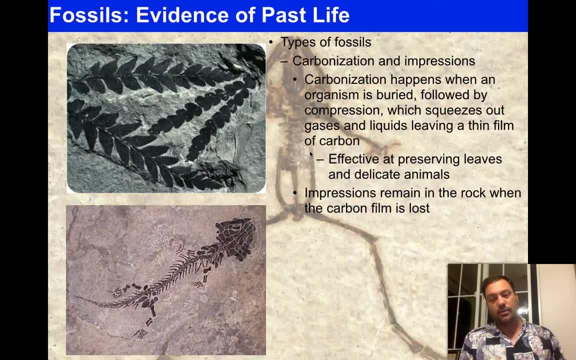 Especially very, very ancient fossils at the beginning of kind of life's history, And of course the impressions remain in the rock when the carbon film is lost, And so here we see a clear reptile impression of a lizard of some sort. 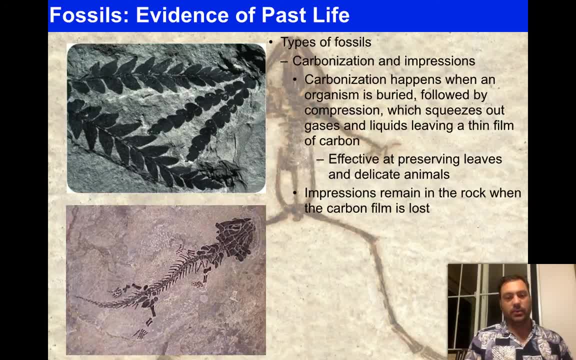 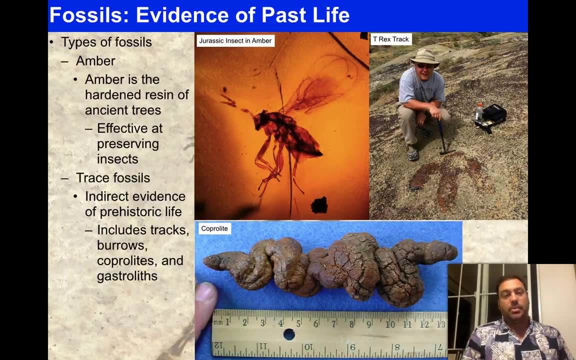 This is, I believe, dates back to the time of the Jurassic, But you get the idea right. This is just carbon. The actual animal is gone, Just the carbon molecules remain. Okay, Probably the most famous of all fossils In the last 20 years are the amber fossils made famous by the film Jurassic Park. 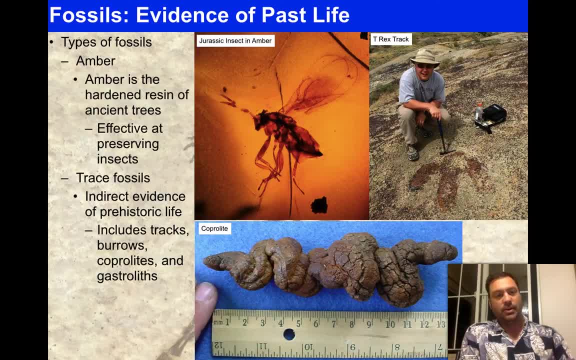 And so I decided to go ahead and put a piece of amber in here. So amber is the hardened resin of ancient trees, right, It's tree sap And it's effective at preserving insects- Really really good In this case. here we see a Jurassic insect in amber. 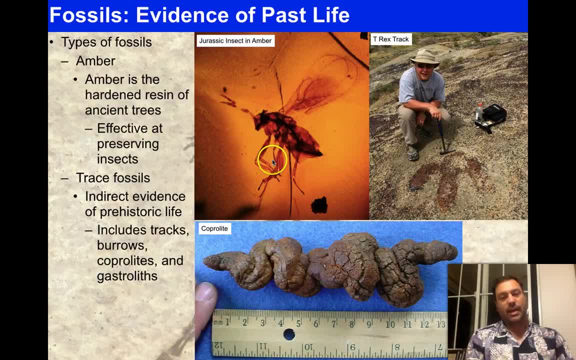 Really, really neat. You can get pieces of amber that have dozens of insects in it And you can study them. There's also trace fossils, which is indirect right. So here we actually see the creature. This is a Jurassic insect. 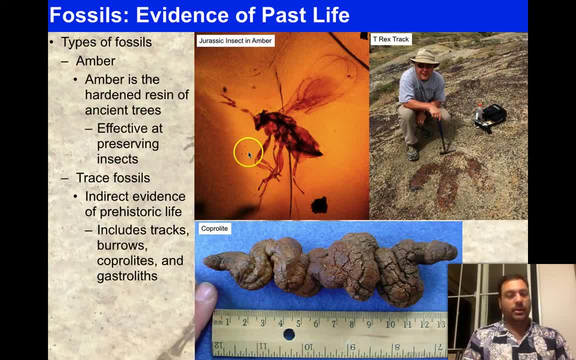 This is, you know, maybe 100 million years old Or maybe older, Sitting here preserved. This insect no longer exists on planet Earth, But here it is in the amber. So anyways, back to trace fossils. Indirect evidence of prehistoric life includes tracks, burrows, coprolites and gastroliths. 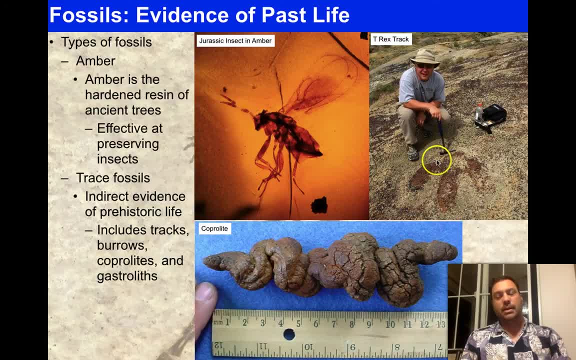 So tracks? here we see a paleontologist. He believes that this is actually a T-Rex track. He gives the odds at better than 50-50 that this is a juvenile T-Rex that was walking through here and left this track. 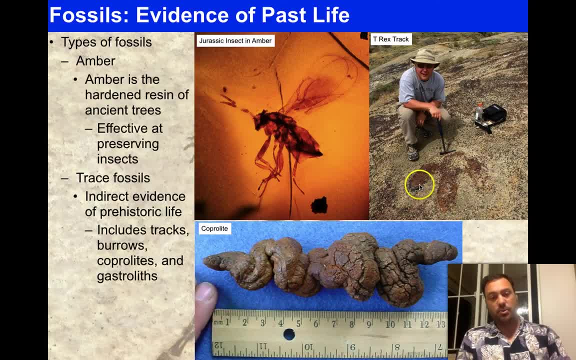 This would have been at some point before 65 million years ago. Coprolite: it is exactly what you think it is. just by looking at it, It is dino-do, That's the best way to put it. The best coprolites we find actually are probably small reptiles that left them. 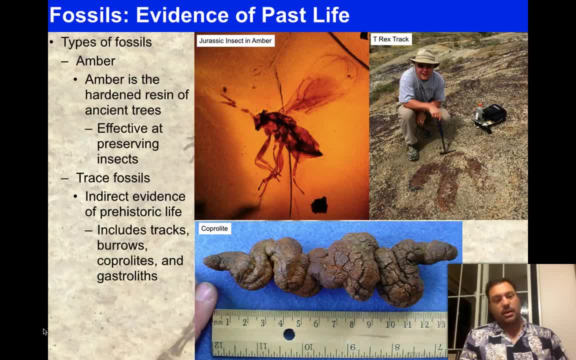 And we can use them to figure out information about their diets. So it's a coprolite Burrows, right? They left holes everywhere they went. We can actually go and look at these burrows And sometimes we can find interesting things in them. 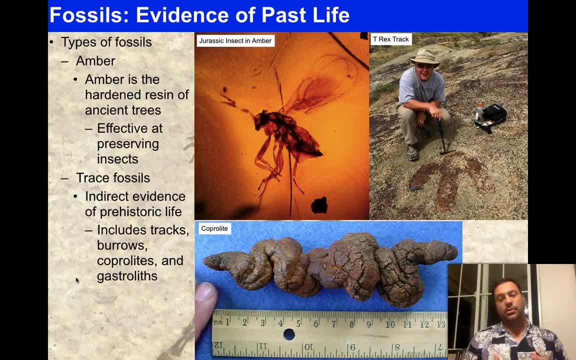 And gastroliths are rocks that a lot of dinosaurs and reptilian cousins of theirs would ingest into their digestive tract to help with the breaking down of different materials, Especially if it was plant materials they were eating. It would help them grind it up kind of in their gizzard, if you will. 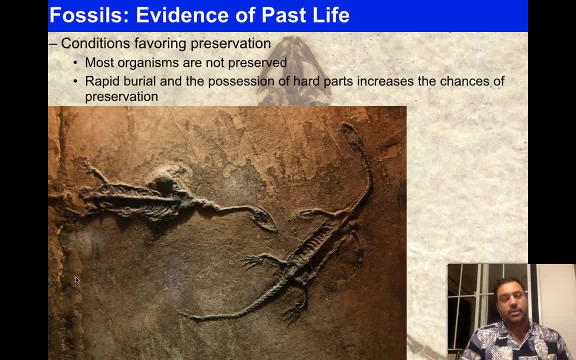 So there are certain conditions that favor preservation. right, Most organisms are not preserved. There's only a few that really are. First off, you need rapid burial and the possession of hard parts to increase the chances of preservation. Another thing that is really helpful is if you wind up getting deposited or you die in an area where your body falls into a zone where there's no oxygen. 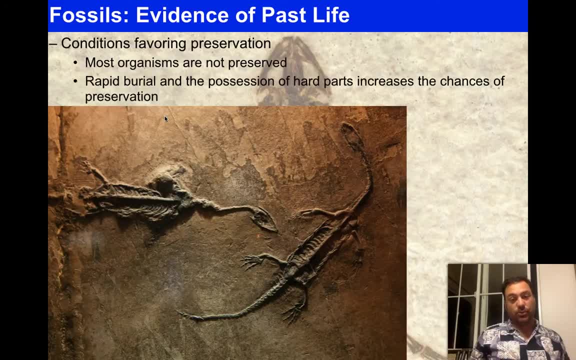 If you don't have any oxygen, there's nothing there that can live to eat you, And so your body gets preserved in the sediment. So here we see, two creatures that have died. These are both dinosaurs- relatively small ones, But dinosaurs nonetheless. 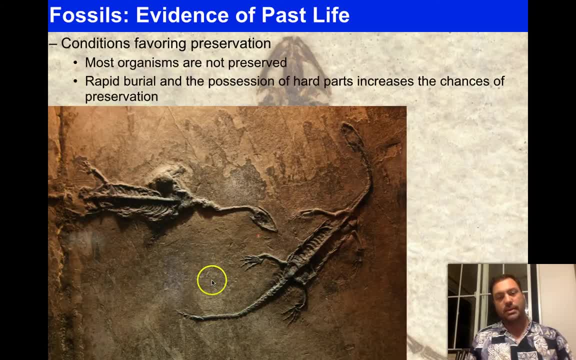 And they've fallen into this sedimentary deposit right next to each other. Really good details, right? You can see the ribs, the spinal cord, the whole thing. Long necks- You can even see the small, intricate details of their hands and feet. 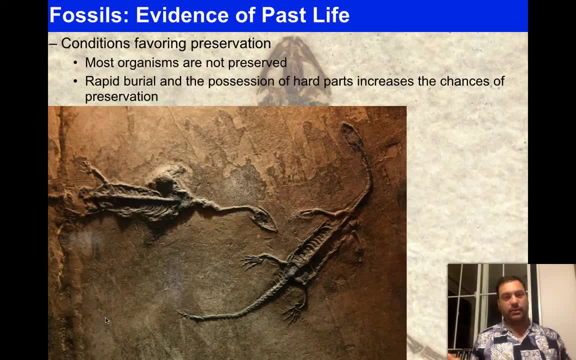 They have hard parts, So it's kind of like everything you need to make sure that you get a good preservation, And this, of course, is some kind of silt or sandstone Or Probably a siltstone, And silks tend to deposit readily and all the time. 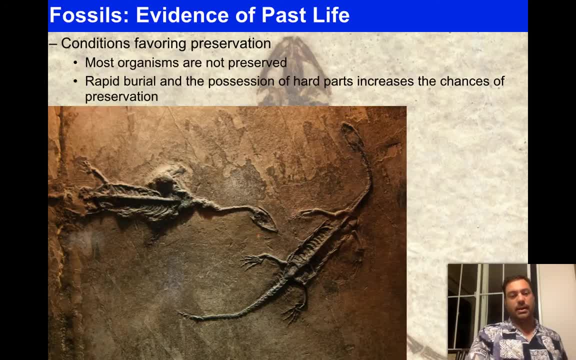 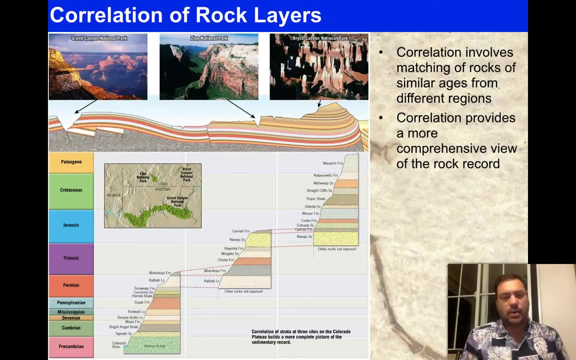 And so, yeah, You get everything you need to be able to deposit these two guys. All right, So that allows us to do some interesting things, right? If we're finding rocks in one place that have certain fossils in it, we can correlate it with rocks that we find in another place. 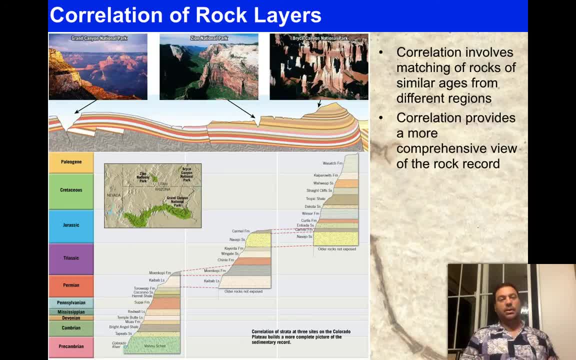 So that allows us to date rocks even further. So, for example, here we can go in the Grand Canyon- We know what the fossils look like- And we can go over here to Zion. We can go over here to Zion. Zion is right here. 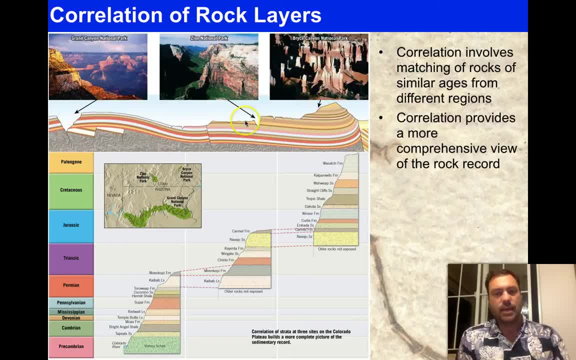 And we can go to Bryce Canyon And we notice that these things stack up nicely. We can look at Bryce And this is what it looks like. It turns out these two formations down here, the Naho Sandstone in particular, correlate very nicely over into the area that we see under Zion. 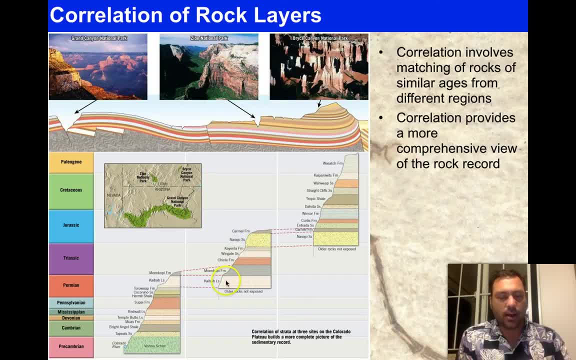 We can go through Zion, through the Kayenta, all the way down into the Kaibab in the Monkope Formation. These two correlate from Zion National Park into the Grand Canyon And so, as a consequence, we get a very large section of sedimentary rocks that we can correlate across this entire region. 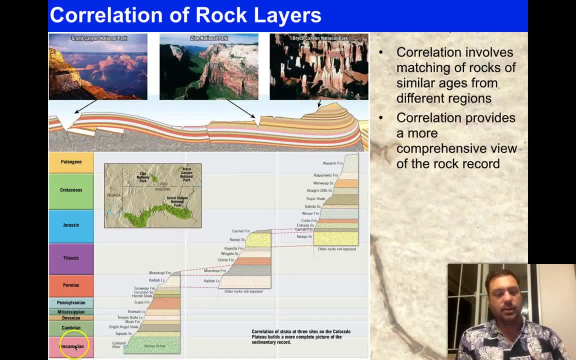 What's really cool is we actually have dates on these Right, So we know from the Grand Canyon what these ages are, all the way up to the Paleogene, which is the youngest period of time that we see expressed in these rocks. Really cool. 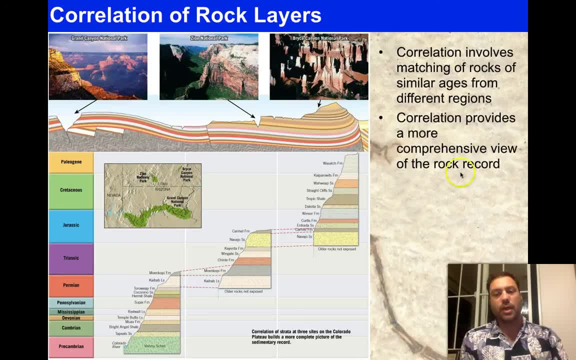 So correlation provides a more comprehensive view of the rock record, something really big, By the way. going from the bottom here all the way to the top, that is something that geologists refer to as basalt. That is something that geologists refer to as the Grand Staircase, because you're basically walking up these rock layers as you go across from Grand Canyon, through Zion, to Bryce Canyon National Park. 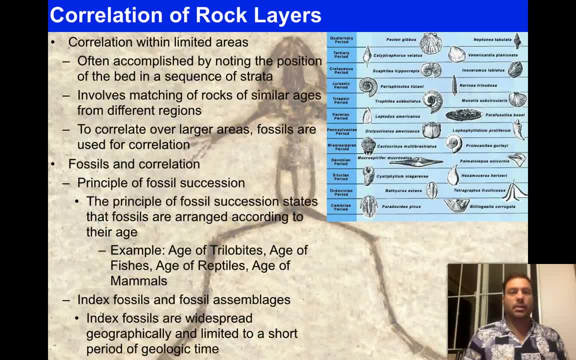 All right, So there's also the. so this would be broad correlations right from all the way across the, you know, northern Arizona all the way up into Utah. We can correlate other things right And the best way of doing this? well, there's several ways we could do this right. 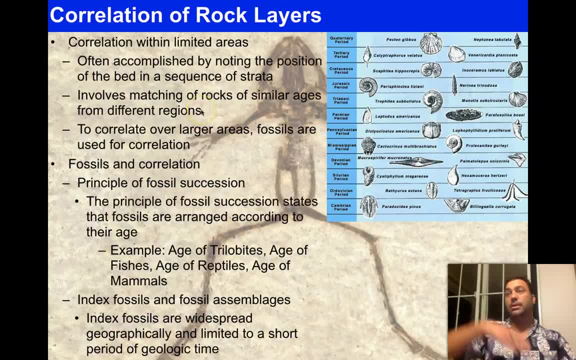 Especially in limited areas. Sometimes they don't extend across right. You get a lake in one place, you get a lake in another place and you don't really know if they're correlatable through environment or whatever. One of the best ways of doing this is to note the position of fossils and to look at the rock strata. 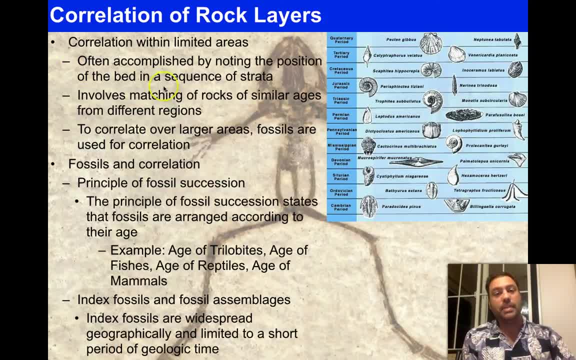 So let's read this here. Often accomplished by noting the position of the bed in a sequence of strata right, So we get an idea of whether they're all about the same age. Involves matching of rocks of similar ages from different regions. 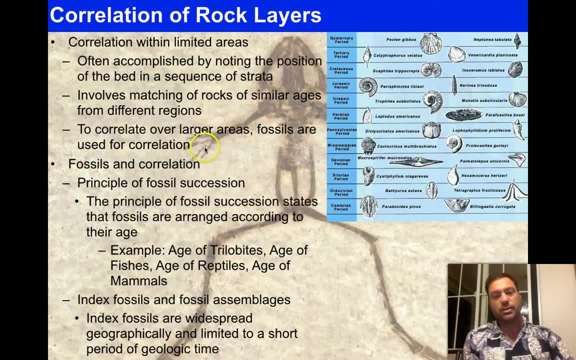 And to correlate over larger areas. fossils are used for correlation. This is the key, And so if we're looking at different, say, ocean basins worldwide, it turns out there's certain fossils that are present at different times. that allows to correlate different areas. 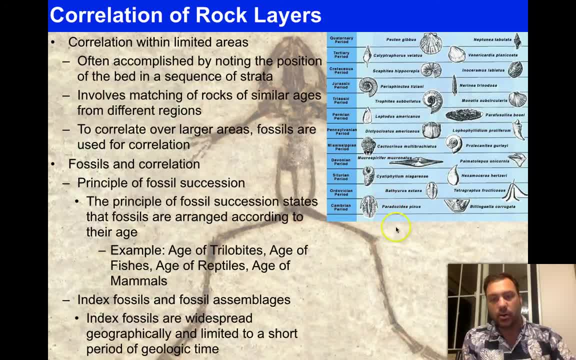 For example, if we're finding- well I don't know- this fossil here during the Permian period and this fossil here during the Permian period, And we find it all over the place, We know that they are at least time correlative. 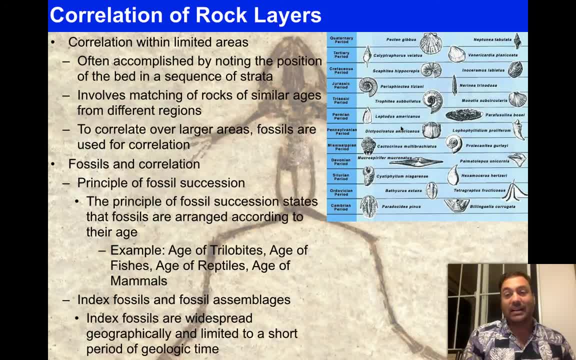 They correlate in terms of time, And so that allows us to be able to know that these were both happening at about the same time. So fossils are really big, So the principle of fossil succession is really important. Things that are really really simple begin evolving right into the Cambrian. 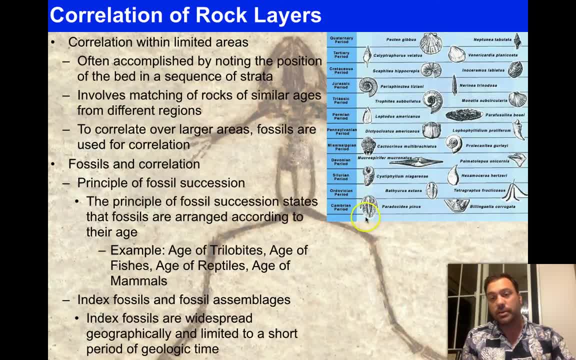 We find really nice things called trilobites, which no longer exist, But they were worldwide along the coastlines back then, And we find things all the way up in the Quaternary Period, such as human beings right That tell us that these were really important. 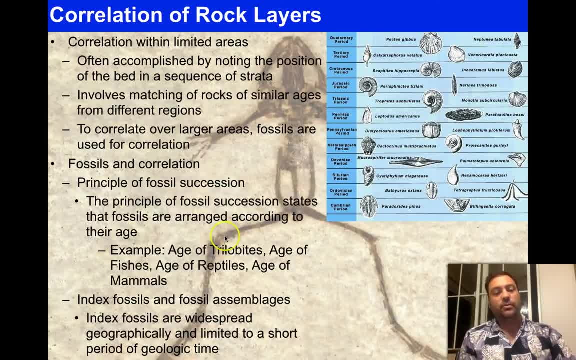 That tell us that these things are of quaternary age. So, for example, we get these things called the age of trilobites, the age of fishes, the age of reptiles, the age of mammals. The age of mammals is the time we live in now. 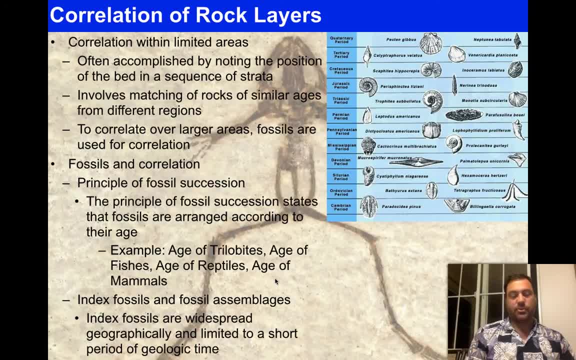 And so if we're finding large mammals, we know we're in the age of mammals. If we're finding dinosaurs, we're in the age of reptiles. So if we're finding the large fishes and the trilobites, we know where we are in that succession. 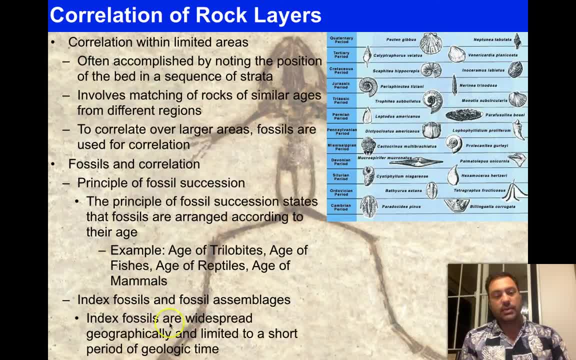 So index fossils and fossil assemblages. So index fossils are widespread geographically And they're limited to a short period of geologic time And that's what this is up here. These are basically the main index fossils. If you find something- for example, this fossil here and we find this fossil here, we know that they're correlated time-wise. 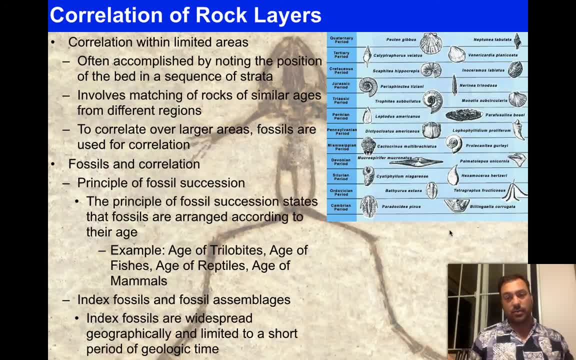 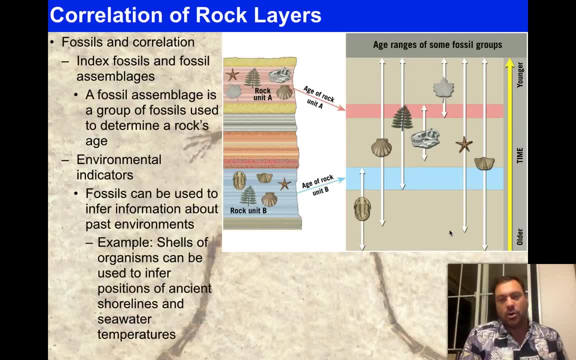 And they probably lived at the same time, or very, very close to the same time, during the Cambrian Period. All right, I know I'm kind of throwing out a lot of jargon, but let's just show how this works, right. 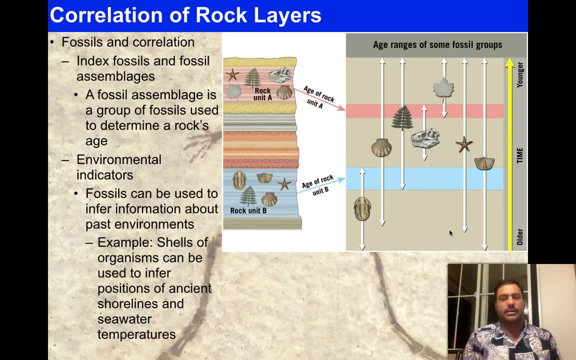 It's kind of better to just show how it works, And you'll get it. So. index fossils and fossil assemblages. So we have a rock right. Here's a rock unit B, Here's a rock unit A, And we want to know its age, right? 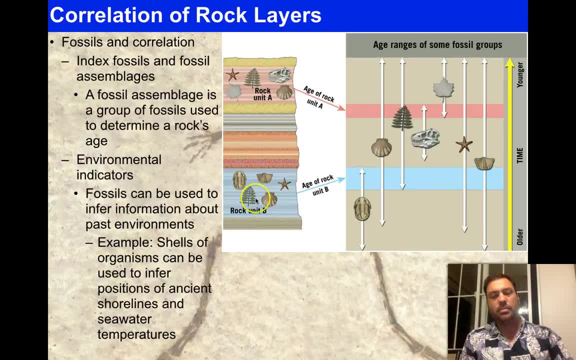 Well, we know that the one on top is younger and the one below is older, But we have some evidence, We have some fossils in here And we can use it to look at the different indexes that are in there, right? So a fossil assemblage is a group of fossils used to determine a rock's age. 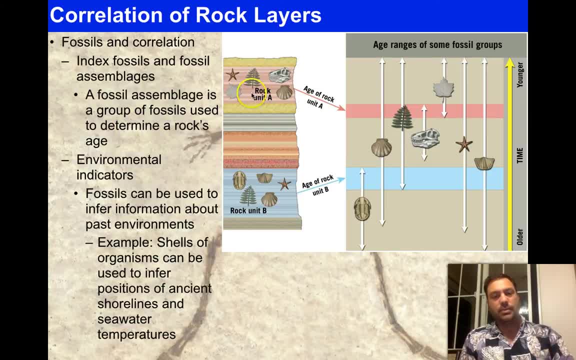 So here we go, Some plants, some leaves. Here's a dinosaur, a scallop and a starfish, And we can go in there and – or sea star, I'm sorry, That's what the oceanographers like to call it. 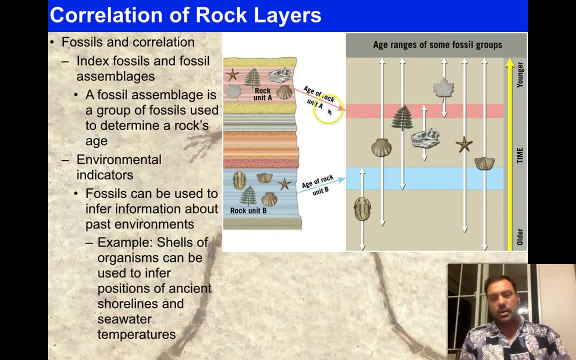 Age of rock. unit A has all of these in here. So we know when these things lived. We know that there's – here we see the scallop, Here we see this – what is probably a fern The dinosaur here, Here's a leaf. 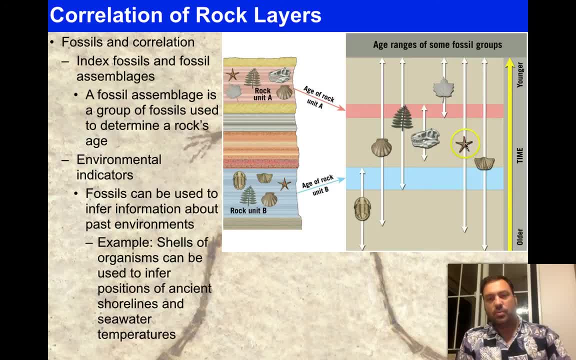 And we find the star, And we find – in this case, do we find this here? I'm looking for it. It's not present up here, but that doesn't mean that it has to be right, Because these other ones exist. 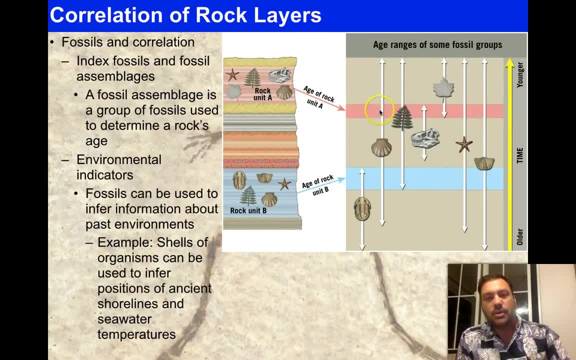 And what we do is we find out where they all lived at the same time. So this lived during this period of time. This lived during this period of time. This lived during this pink period of time. You'll notice that it can't be any older than that, because if it was any older, we wouldn't find this leaf anymore. 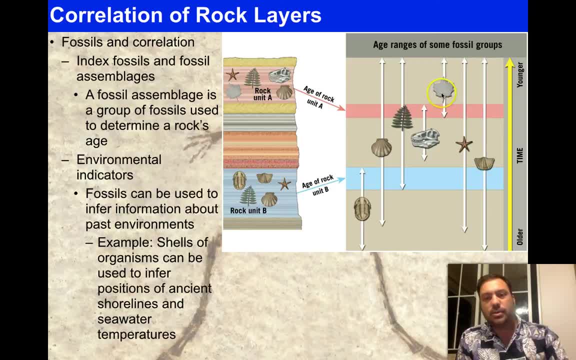 That leaf right here only exists during this period of time, So this is one bracket. The dinosaur here had – the T rex head had to be – had to be in this time, So we know that it had to exist during this pink period of time. 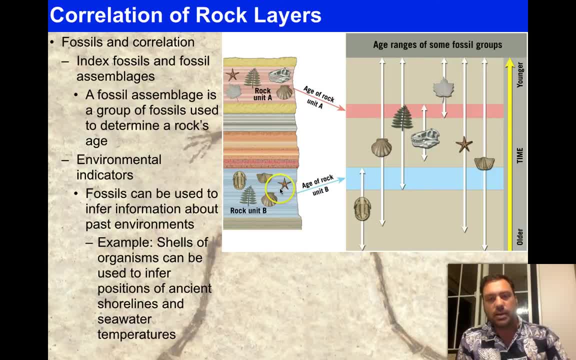 Same thing is true down here, right, We find the starfish, But instead of finding the leaf right, instead we find the trilobite. So we know that the trilobite lived only up to this point and this leaf only lived down to this point. 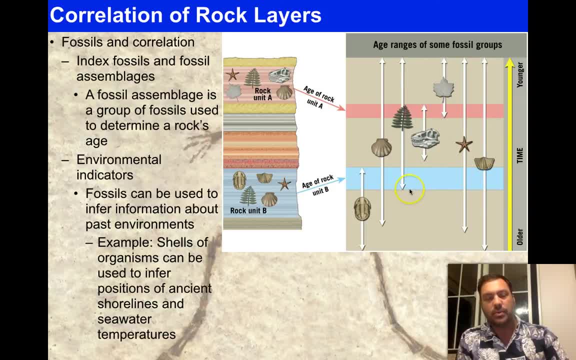 So this is the only thing that matches all of the data that we see there And that allows us to get an age relative on this. So this might be Cambrian, whereas this up here might be belonging to the age of mammals Or, I'm sorry, to the age of reptiles, because there's a dinosaur in it. 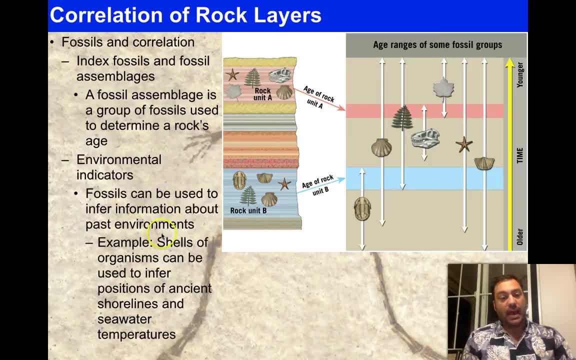 So fossils can be used to infer information about past environments, All right. so this is kind of almost so obvious, right? Shells can be – shells of organisms can be used to infer positions of ancient shorelines and seawater temperatures, Even just on the first order, right? 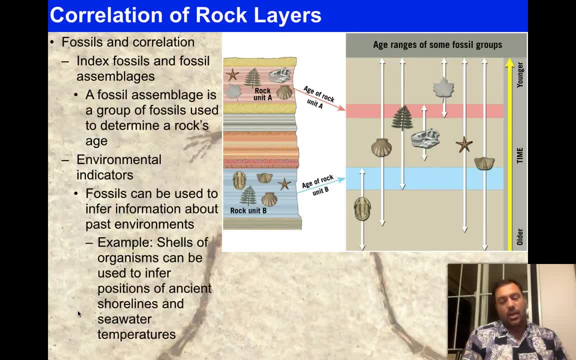 If you're finding a T rex head, you're not in the deep ocean. If you're finding scallops, you're probably in the deep ocean. If you're finding scallops, you're probably somewhere near the coastline. If you're finding ferns, you're probably in some type of marshy environment or coastal environment- things like this right. 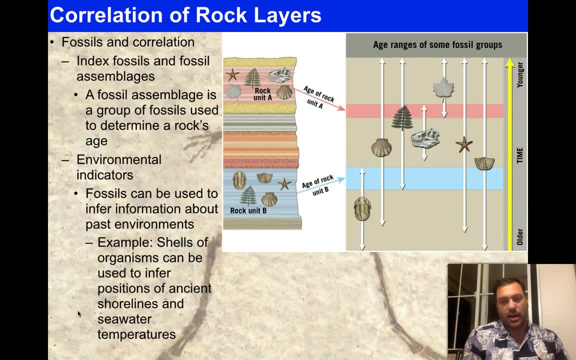 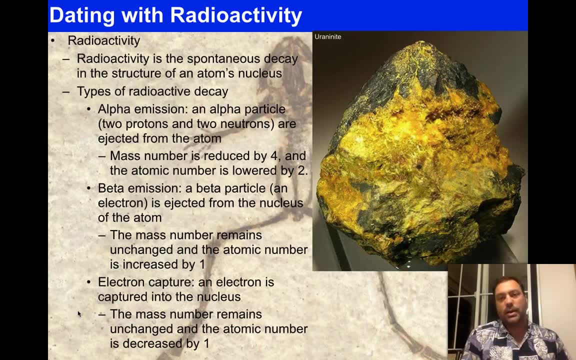 You're not going to expect to find a bunch of vulture bones and fossils in the middle of the ocean. right? That's the environmental indicators, All right. so we kind of got the idea that there's these animals that live at different times. 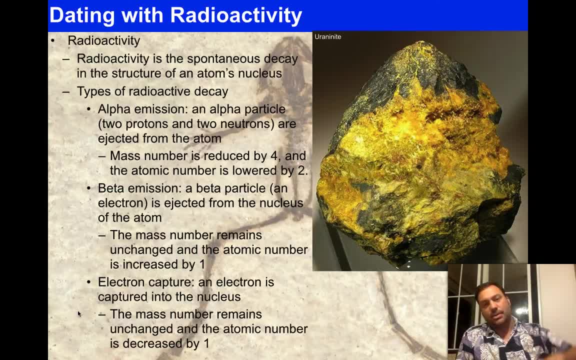 They evolved into different times at different times, I should say. So how do we put dates to it then? The answer is that we figured out how to do this using radioactivity. That's the main way that we do it. I wish there was a more sophisticated way, but this is probably 98% of the ways that we do our absolute dating. 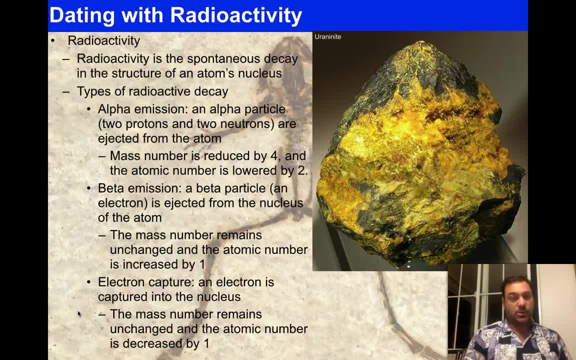 We get a real number and say how old something is, It's using radioactivity. So radioactivity is the spontaneous decay And radioactivity is the structure of an atom's nucleus. We actually talked about the structure of the atom at a much earlier lecture on the principles of matter and how it operates. 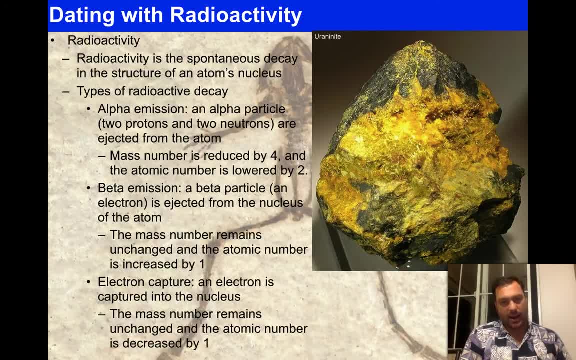 And if you have any need to go back, you should go back, find that lecture and review that before we go ahead. if you don't remember the structure of the atom, So I'm going to assume that you still have that fresh in your mind or that you have some fresh experience with it. 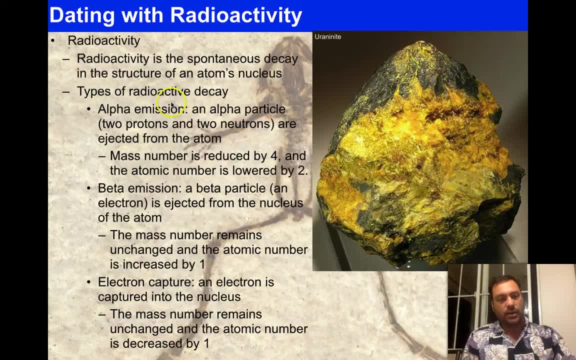 So the types of radioactive decay, there's several. The alpha emission, so in other words the decay in that structure of the nucleus. we can see an alpha emission which is an alpha particle, So two protons and two neutrons are ejected from the atom. 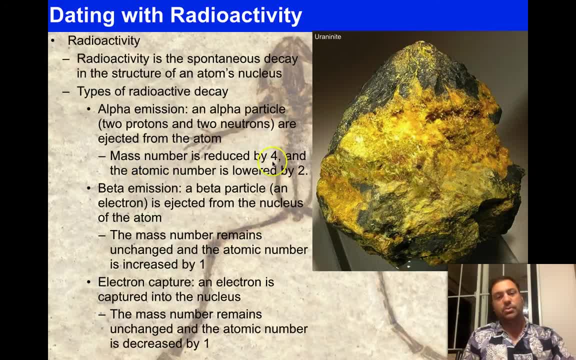 They just come out, And so happens the mass number is reduced by four and the atomic number is lowered by two, because we have two protons that are lost in the process. But we add the number of neutrons and protons. That tells us the atomic mass. 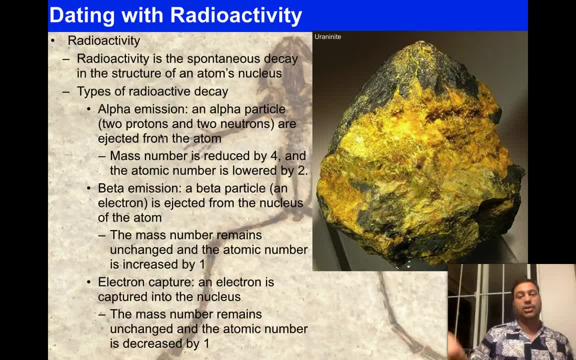 So the thing gets lighter by four and the element changes by two down on the periodic table. So beta emission is a little different. So this is where an electron is simply ejected from the nucleus, And this usually happens at the expense of a neutron. 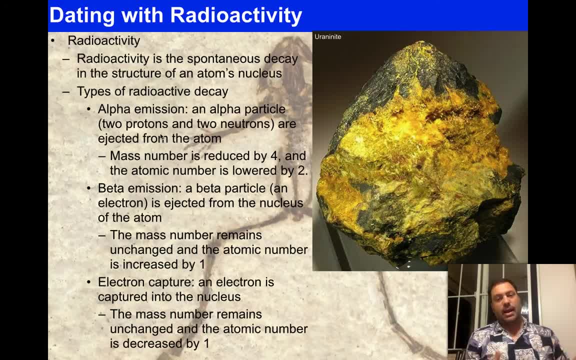 So we lose an electron by shooting it out of the nucleus, usually from a neutron. So the mass number remains unchanged- right, It doesn't really change, But the atomic number is increased by one. Why? Because that neutron, by virtue of shooting out the electron, becomes a proton. 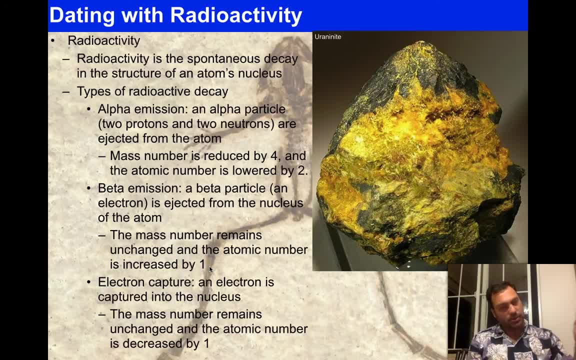 Right, Remember. if this is confusing to you, please go back and review that lecture. And lastly, electron capture. An electron is captured into the nucleus, So this is where it's absorbed. It's the exact opposite of the beta emission. 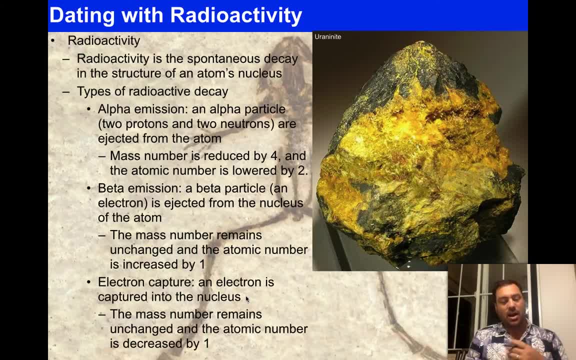 It's the electron capture. So in this case, a proton takes on an electron, It fuses and it becomes a neutron. So the mass number will still remain the same. It's not going to change. The electron number will be decreased by one. 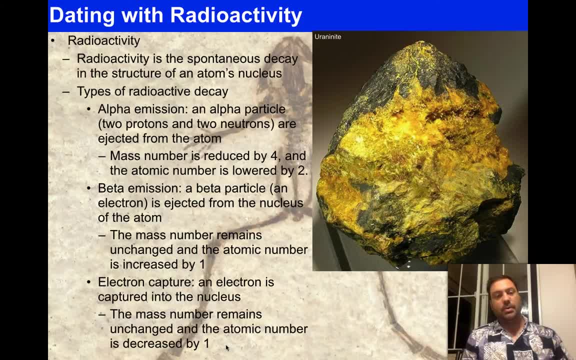 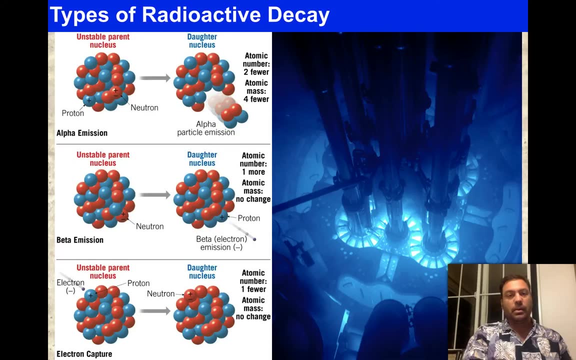 Why? Because the proton is now a neutron And anyway we have the mineral uranite here. This is a primary uranium ore And uranium is one of the lead elements that we use to date ancient rocks. So here we see this kind of exhibited directly. 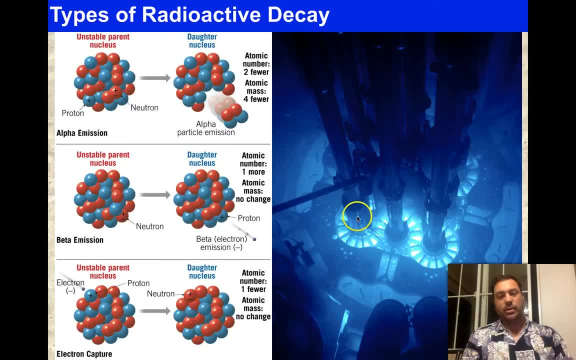 This is a nuclear reactor. We see kind of the glowing of the light is due to the emissions, The emissions going through the water, this water here, and it's making the water glow blue. It's kind of cool. So, anyways, here we see this unstable parent. 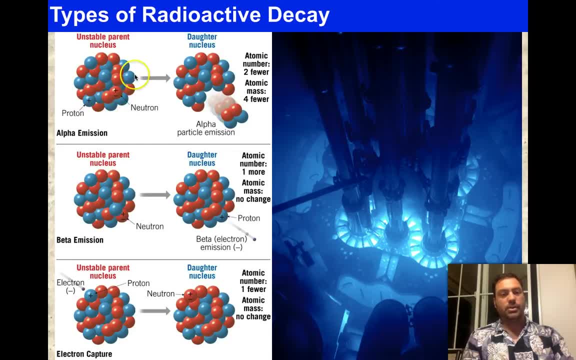 Basically, we have a proton-neutron situation here And we just take part of it and we just shoot it out And that's going to change the nucleus. It's going to become one atom to a different kind of atom. This is actually a helium atom that's emitted. 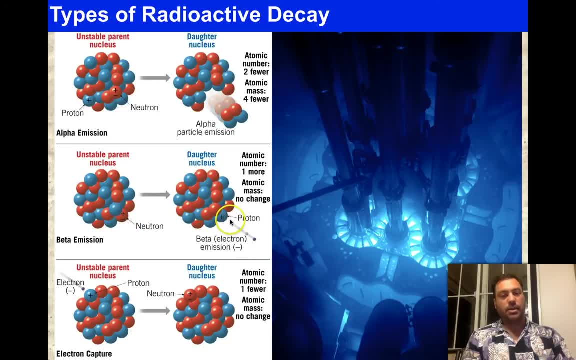 And the beta emission. the neutron here shoots out an electron and it becomes a proton. So that changes the nucleus again To something different. So it becomes a different element. And the same thing here, right, The electron comes in, combines with the proton, becomes a neutron and we wind up with a new nucleus again. 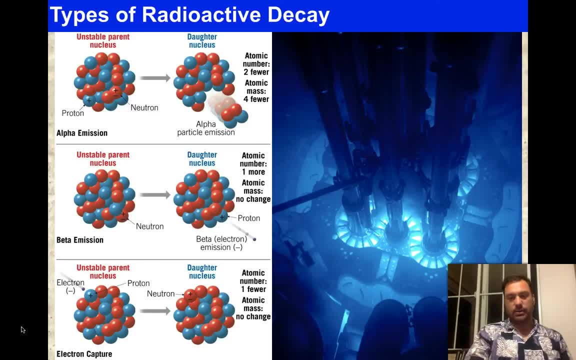 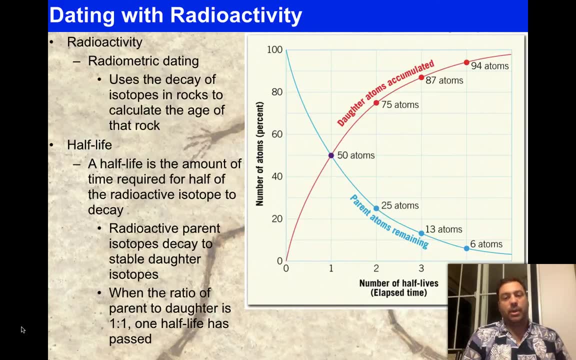 So these are the different kinds of radioactive decay that we can experience. Now the really cool thing about this process in radioactive decay is that it happens at a statistically predictable rate, Right The amount of decay that will happen. So radioactive decay, Radiometric dating, is completely dependent upon this idea. 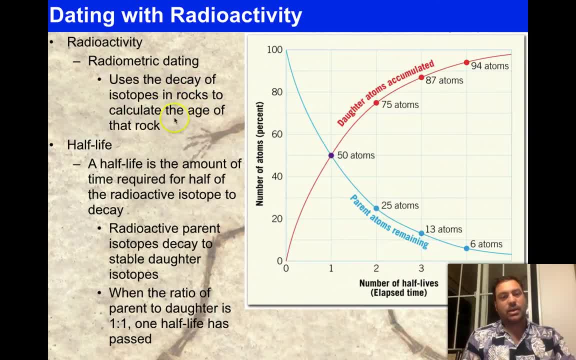 So it uses the decay of isotopes and rocks to calculate the age of that rock, And so we wind up with something called a half-life. A half-life is the amount of time required for half of the radioactive isotope to decay, So we might have 100 atoms in this case. 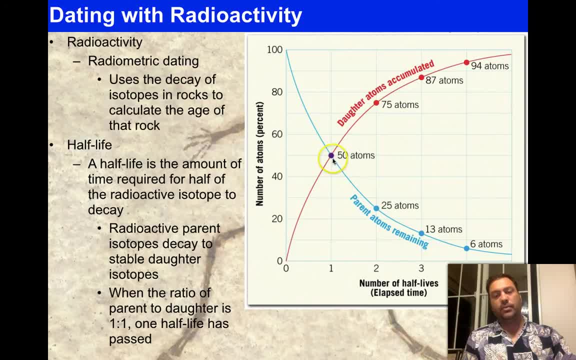 And over some period of time we're going to wind up with 50. So we can put a dot right there And that's our first half-life. Now the second half-life is kind of cool because that 50 is a second half-life away. 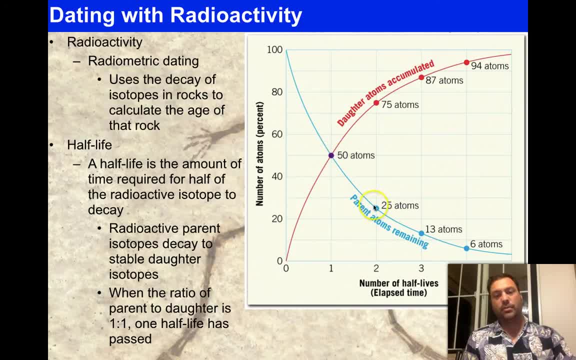 So it's the same amount of time when we go from 50 to 25.. So it doesn't go from 100 to 50 to 0. That 50 becomes 25.. And then it goes half again, That 25 becomes 13.. 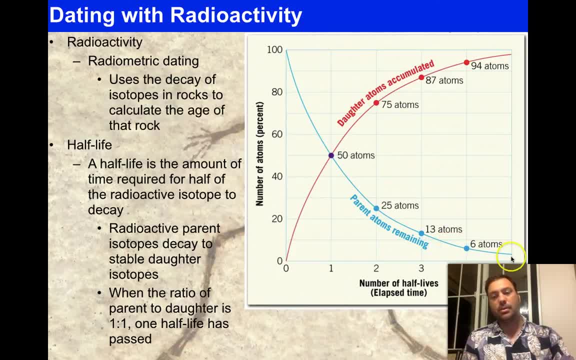 That 13 becomes 6.. That 6 is going to become 3.. That 3 is going to become 1 and a half, And so on and so forth, And of course, the number of daughter atoms that we're going to be accumulating while we do this also goes up by the same amount. 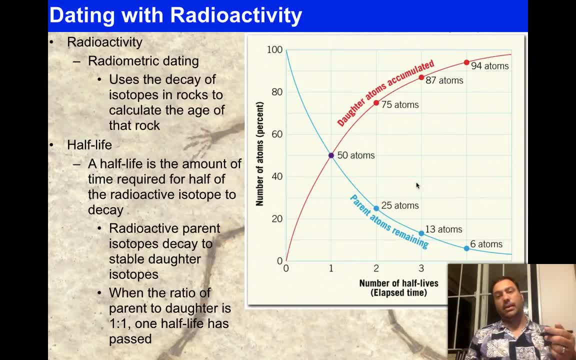 Right. So one is forming at the expense of the other. So the daughter atoms are accumulating while the parent atoms are being destroyed. So radioactive parent isotopes decay to stable daughter isotopes. That's the idea. When the ratio of parent to daughter is 1 to 1, one half-life is passed. 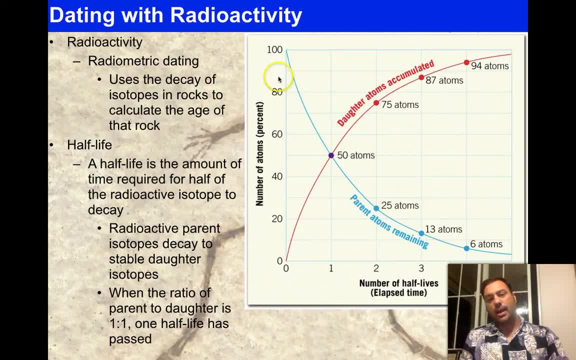 So if we're looking at something that originally had 100 atoms of, say, uranium and now it only has 25 atoms of uranium and maybe 75 atoms of daughter material- maybe lead is the main thing- then we know that two half-lives have gone by. 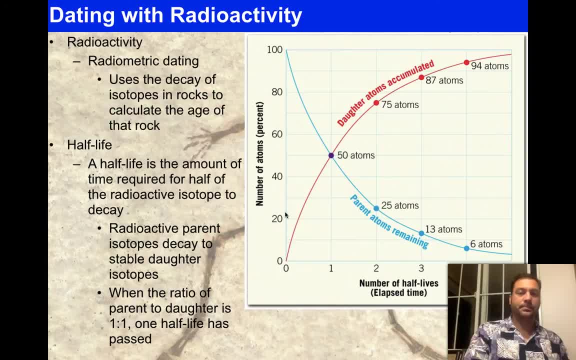 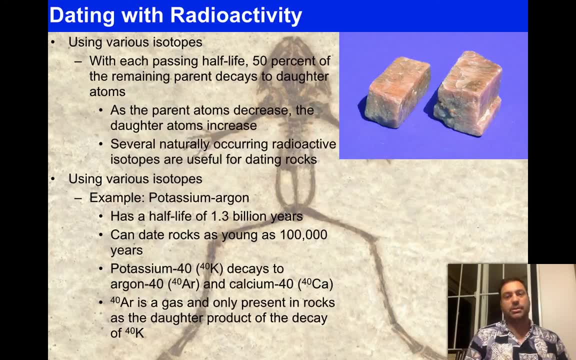 And so we can use that to figure out how old the rock is. That's the idea. So with each passing half-life, 50% of the remaining parent decays to another atom. That's what we just discussed. As the parent atoms decrease, the daughter atoms increase. 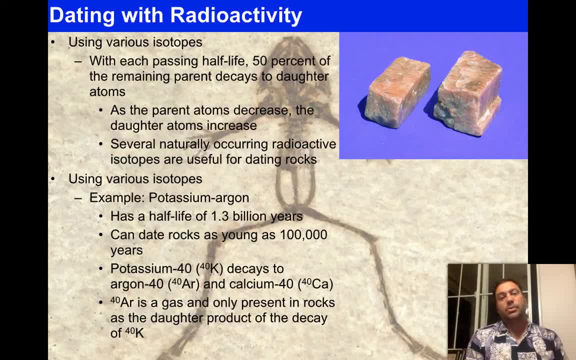 So one goes up, the other, one goes down. Several naturally occurring radioactive isotopes are useful for dating rocks, And we're going to talk about those. One of the main ones that we're going to be talking about, which we'll kind of briefly bring up, is potassium to argon. 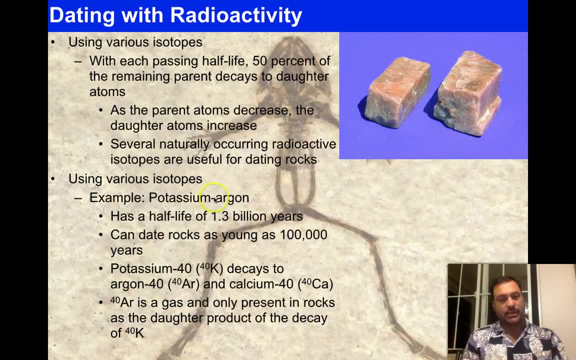 This is a really useful one. It's common. Potassium decays into argon in K-spar and potassium feldspar. This is one of the most common rocks in continents. It's found in a lot of sandstones And it's a really hard rock. 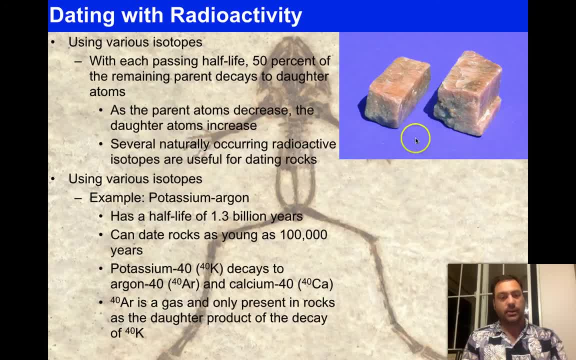 And it stands up to weathering very well, or mineral I should say. So this is really kind of cool. It has a half-life of 1.3 billion years, So that's kind of cool. In terms of Earth history, it's about 25% of Earth history is the half-life. 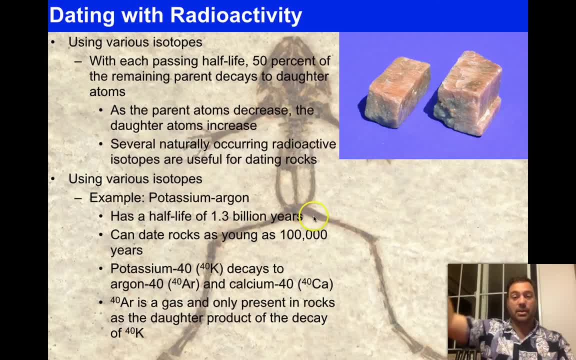 So that means that it has some good resolution. to go beyond that, As long as we have several half-lives in, we can go three or four half-lives and we can figure out how old these minerals are. It can also date rocks as young as 100,000 years. 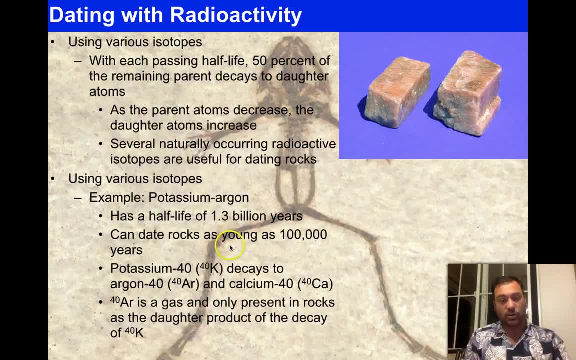 So it can go the other way, right, It can go very, very young as well. This is a really cool process. There's some other ones right: Potassium 40.. That decays to argon 40.. 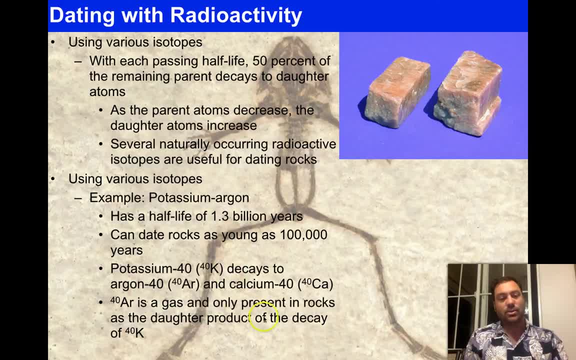 And calcium 40. We see both of these And argon is a gas and only present in rocks as the daughter product of the decay of potassium. So essentially what we see here is that we can go through. I can say: hit this with a laser at some special place right on the crystal, where I know I have a good crystal. 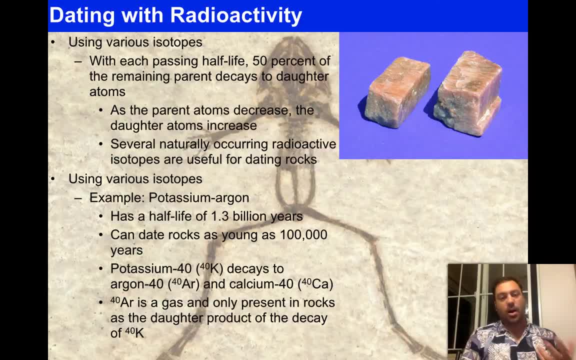 I hit it with a laser and I blast it And I measure the amount of argon that comes out of it. And I know that that argon had to have come from potassium, because potassium feldspar doesn't use argon to form. 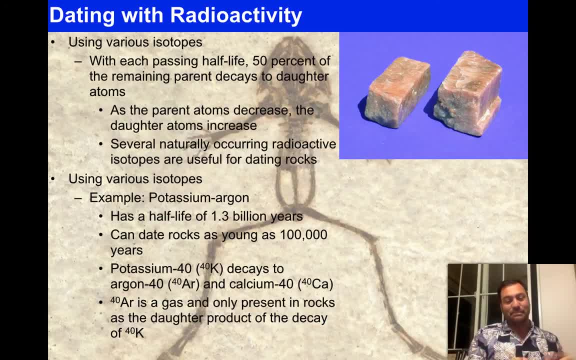 Potassium. feldspar makes potassium, It uses potassium. It's through the radioactive process, it's through the decay process, that argon is produced, long after the mineral is formed. So it's trapped in that mineral And so we're able to go through and measure the amount of argon that we find in this rock. 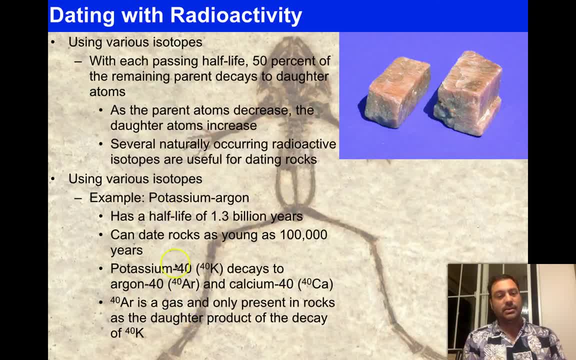 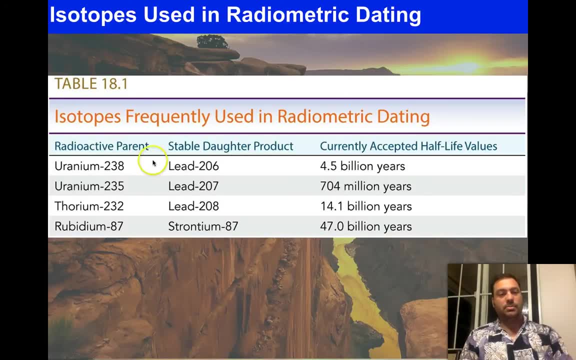 And that allows us to get that nice date. This is a really cool technique. So, anyways, here we see potassium feldspar up here. Here's some other ones. Uranium 238.. This is a common uranium. It's the most common one to lead 206.. 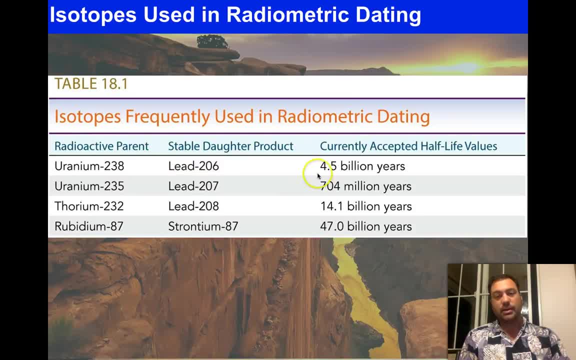 This is the common decay Stable daughter product. It takes about 4.5 billion years, So it's actually pretty stable. Radioactivity in uranium 238 is fairly low. When we compare that to other things, it's not too bad. 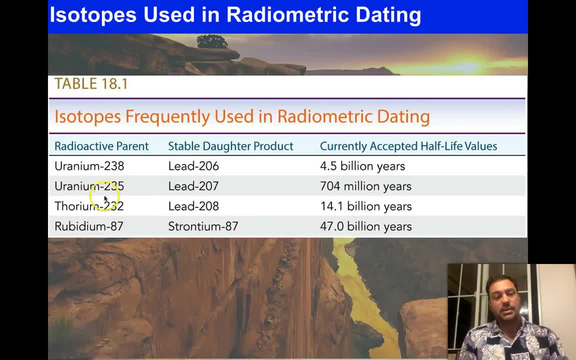 Uranium 235,, which is really famous because this is the variety that is used in nuclear weapons. it decays to lead 207.. And that takes a shorter period of time: 704 million years. Thorium 232 to lead 208,- 14.1 billion years. 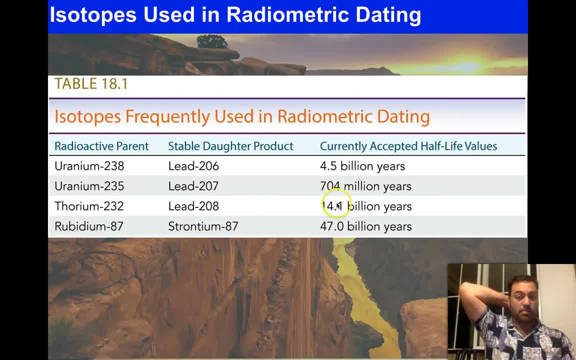 This is almost the age of the universe, right. as we know, The Big Bang was about 13.7.. Rubidium dystrontium. look at this one: 47 billion years is the half-life. That's longer than the accepted age of the universe by far. 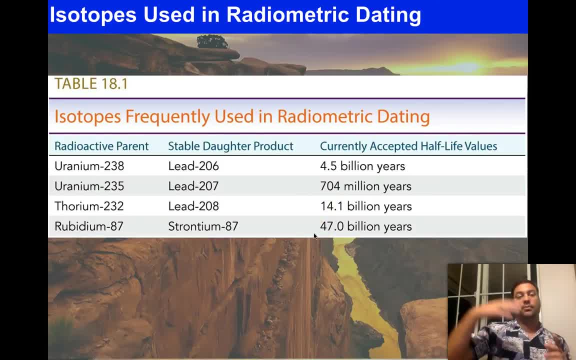 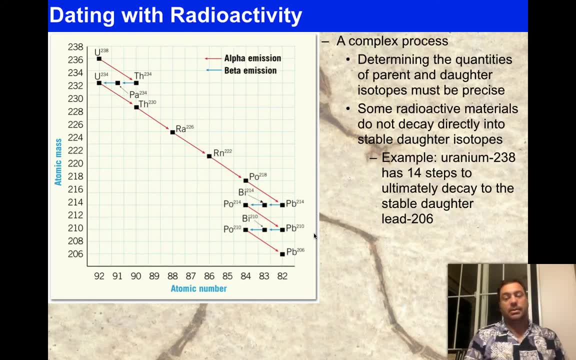 Even this is older than that, So we have the ability to look at information way back In geologic time. This is not always a straightforward process. I'm talking about uranium 238 going to lead 206.. It turns out that uranium 238 to lead 206 is actually 14 steps. 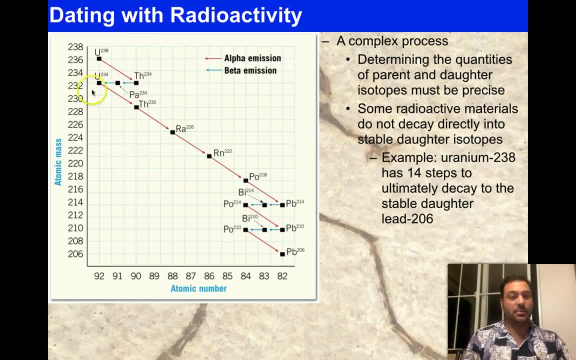 It goes uranium to thorium, back to uranium, Thorium, radium, radon polonium, lead Polonium, again lead polonium and then back to another isotope of lead. So it goes from lead 214 to 210 to 206.. 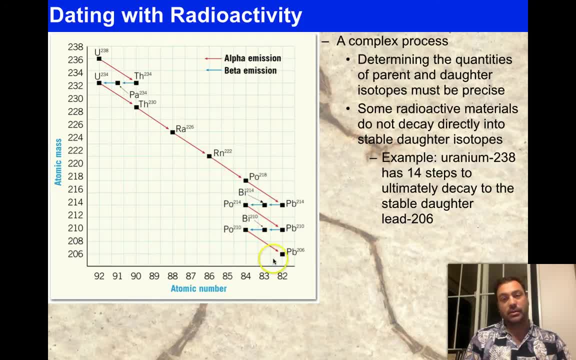 It's a 14-step process if I was to go through all of these things, So it can be a little complicated, right? You're going to find these other things in your rock too, And this could actually be helpful. A lot of geologists are now looking at decay ratios in rocks between 238 and, say, radon 222 or radium 226.. 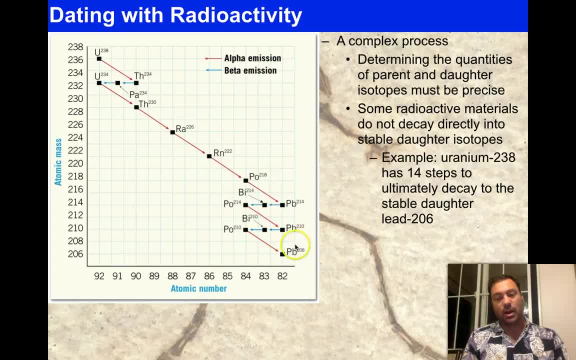 But by far the best for dating the rock itself is 206.. This is. Some of these isotopes up here are useful for figuring out other bits of information, such as uplift rates or how fast rocks cool off. things like that, All right. 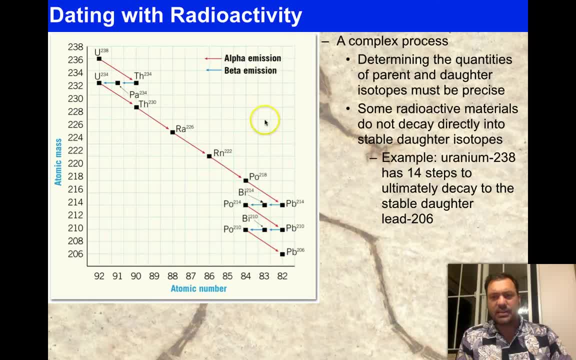 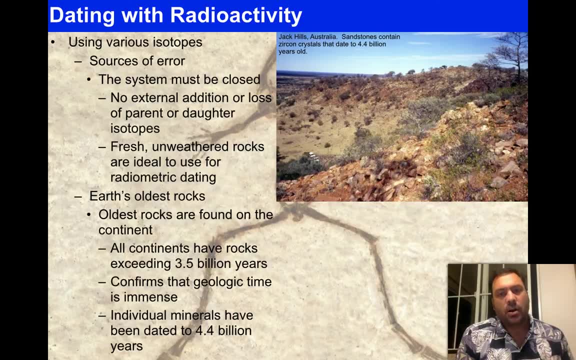 I'm kind of digressing on that, But you get the idea. This is not always a real simple thing. Okay, There are other isotopes that we can use. I'm not going to get into them. We'll talk about carbon either this lecture or next. 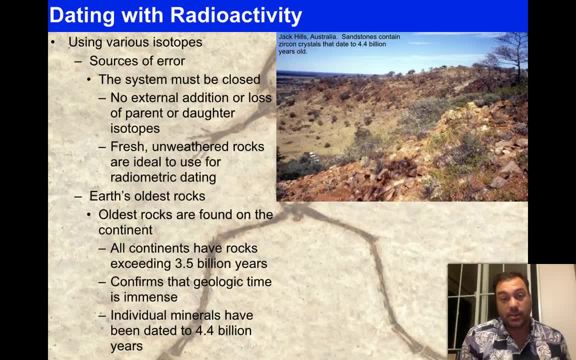 Carbon-14, which is used for dating things in the modern era. But there's all kinds of sources of error, right? The system must be closed, right? You can't have a bunch of fresh argon flushing through your potassium-argon crystal or you get all kinds of mistakes, right? 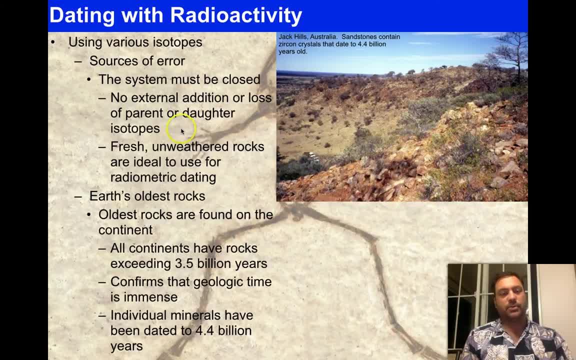 No external addition or loss of parent or daughter isotopes. So fresh water is a- I'm sorry, Groundwater is a real problem. if it's flowing through rocks It can cause things to change. Fresh, unweathered rocks are ideal for useto use for radiometric dating for that purpose. 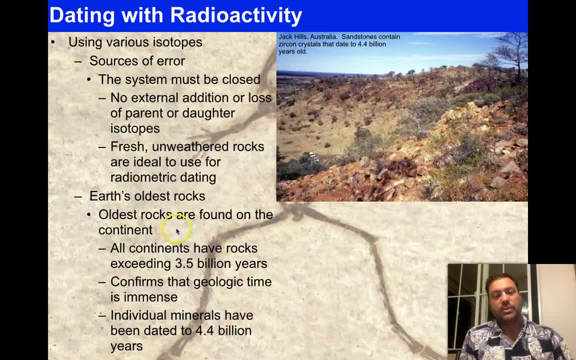 So Earth's oldest rocks are found on the continents right. All continents have rocks that exceed 3.5 billion years. whether it be Greenland, Canada, South America, whatever You go to any of the major continents, you're going to find at least a portion of it somewhere that's 3.5 billion years old. 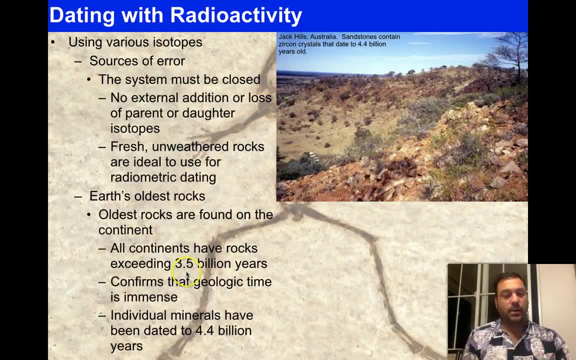 So the continents are quite old, At least the starts of it, the very hearts, And it confirms that geological history, And it confirms that geologic time is immense, Very, very old. The Earth, as we've discussed, is over 4 billion years old. 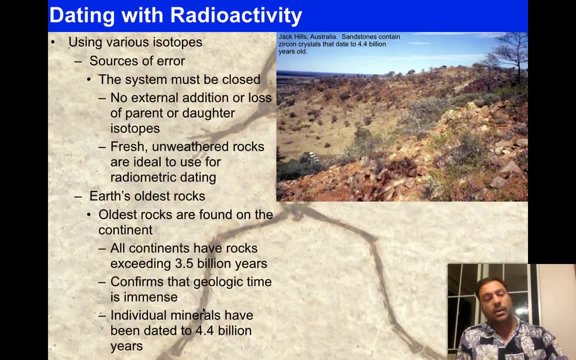 You know, 4.6, 4.55 billion years old And individual minerals have been dated to 4.4 billion years. We have never found anything older than that. As we've said before, and I've said many times, we assume the Earth to be about 4.55.. 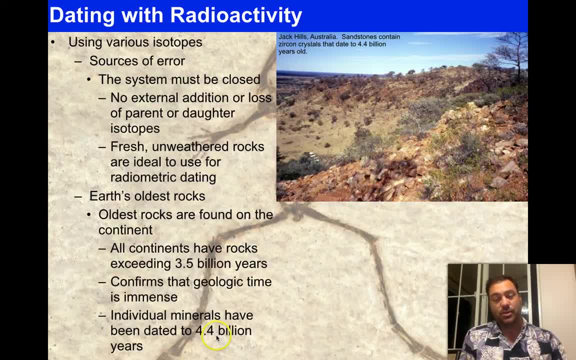 So this is about 100 million years after the creation of the Earth- Less than 200 million years for sure. We have found individual minerals, And this is where we find them: A place called the Jack Hills in Australia, where we have sandstones that contain zircon crystals that date to about 4.4 billion years old. 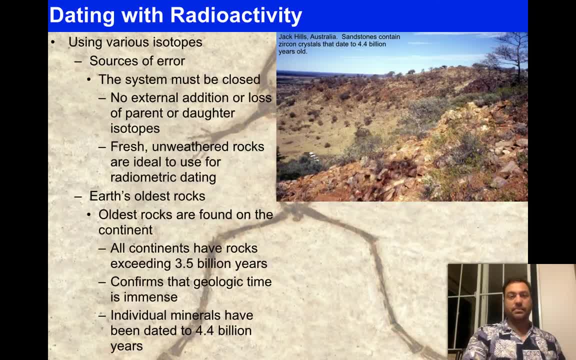 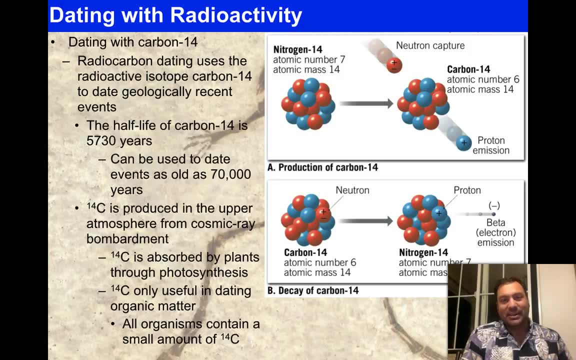 That's right after the formation of the Earth. We find zircons Really really neat. Oh, here it is. actually I wasn't sure if it was in this slide or the next one, But anyways, we're going to talk about carbon-14.. 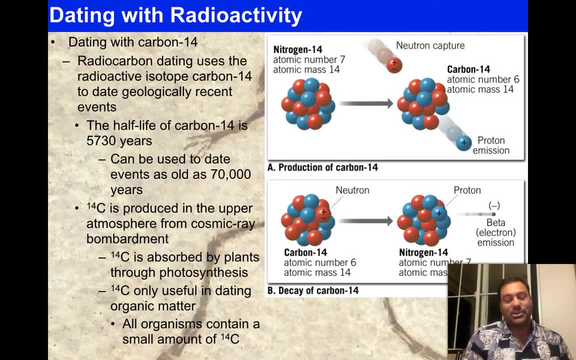 So carbon-14 is really cool. It's used in archaeology. It's used in very young archaeology. It's used in very young geologic studies, or to say, young rock or young processes, geologic studies. So radiocarbon dating uses the radioactive isotope carbon-14.. 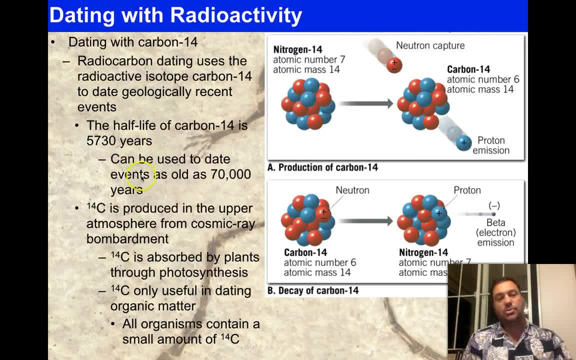 Half-life is 5,730 years. That can be used to date events as old as 70,000 years. right Beyond 70,000 years, there's so little carbon-14 left that we don't see it anymore. So essentially, this is the chemistry. 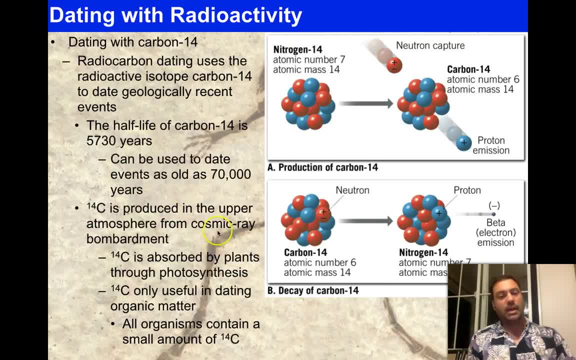 C-14 is produced in the upper atmosphere from cosmic ray bombardment. So we have basically here's nitrogen-14, which is pretty common. There's some neutron capture, that happens. So basically a neutron comes in and it pushes out a proton. 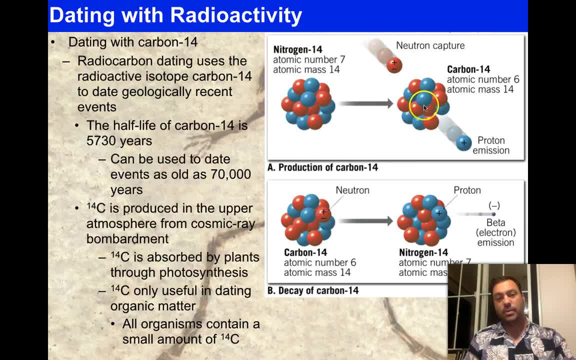 So a proton emission And we've wound up with a carbon-14.. It's radioactive. This is radioactive carbon-14. So the carbon-14 is absorbed by plants through photosynthesis. Why? Because carbon-14, just like carbon-12 and carbon-13, has the same amount of carbon-14. 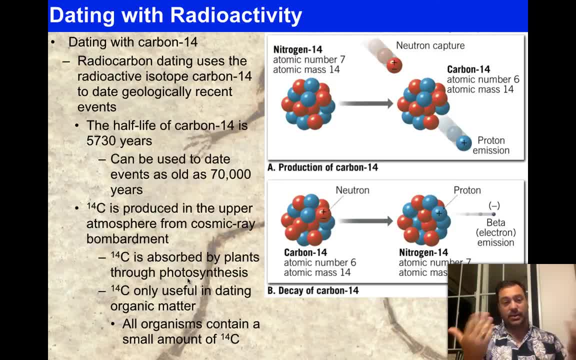 Carbon-13 has the same chemistry. The plant doesn't know the difference and it just takes it in. So C-14 is only useful in dating organic matter. as a consequence: right, We have to have plants or wood or something like that in there. 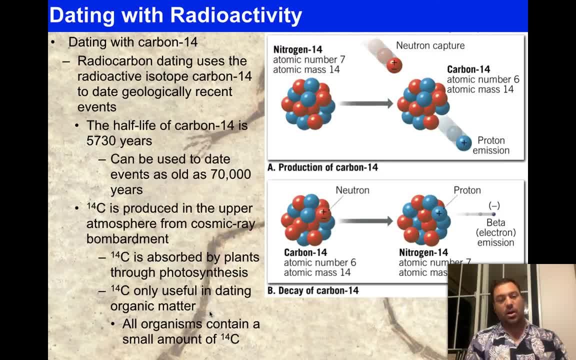 Rocks don't absorb carbon-14. And all organisms contain a small amount of C-14, including you. You're watching this little lecture right now and, yeah, you're breathing in C-14, into the carbon, Or you're consuming plants. 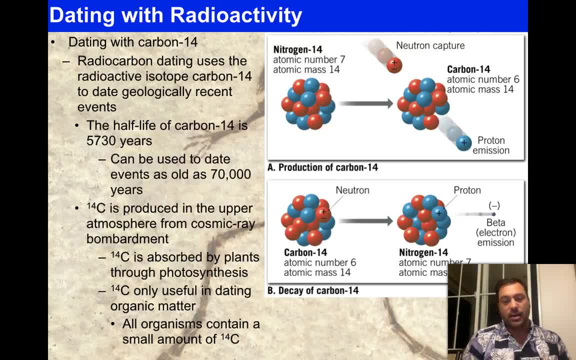 Plants that have absorbed C-14.. And so, as long as you're alive, you're consuming new C-14.. You're keeping that reservoir of C-14 up to date. It's when you die that everything starts to break down and you're not consuming any more C-14. 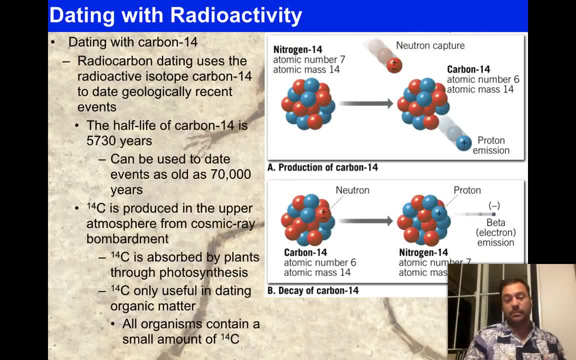 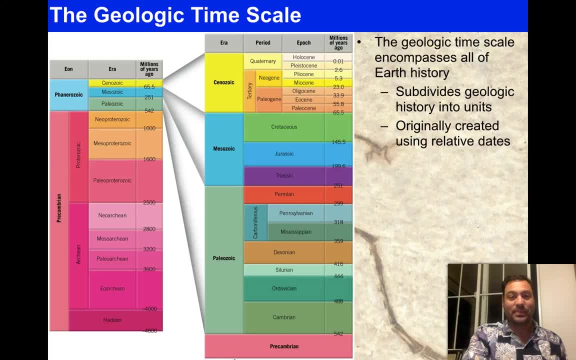 So your radiometric clock is started at that point when you're dying. So that's the cool thing about C-14 is that it doesn't necessarily measure when you were born, but it does tell you when you died. All right, So we can now put together what we think of, or what we see as the geologic timescale. 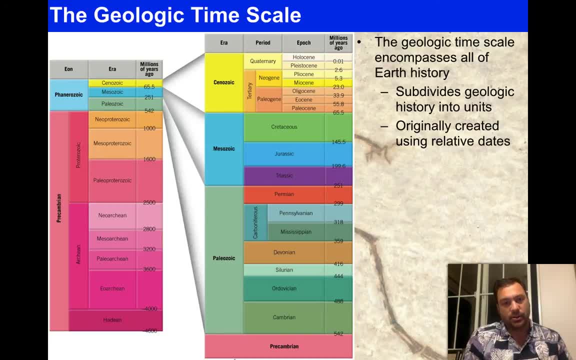 So the geologic timescale encompasses all of Earth, history, Everything. There's a lot of stuff in it. I wish I could go through each part of it. This is actually a bigger. there's a larger class that deals with the geologic timescale, called historical geology. 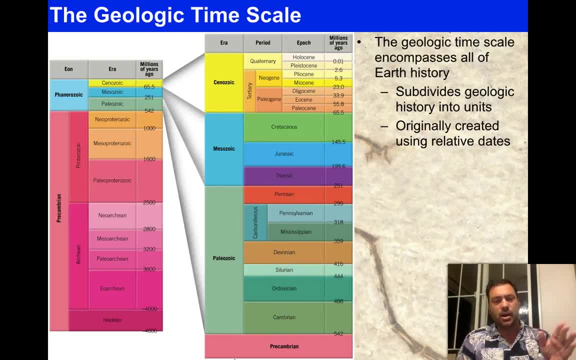 We talked about that in lecture number one. There were two branches of geology: the physical, which is the course that you've been taking, and the historical geology, which is the course that you've been taking. This is the course that is usually taken by people who have a deeper desire to learn more geology. 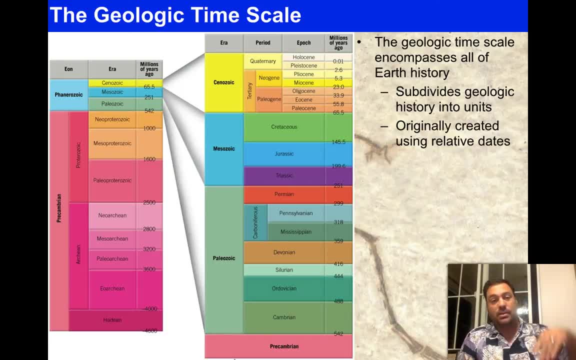 And they learn the geologic timescale and what happened throughout Earth history as they go through it. Let's go through this really quickly. So it subdivides geologic history into units and originally created using relative dates. We didn't have the radiometric dates until much, much later. 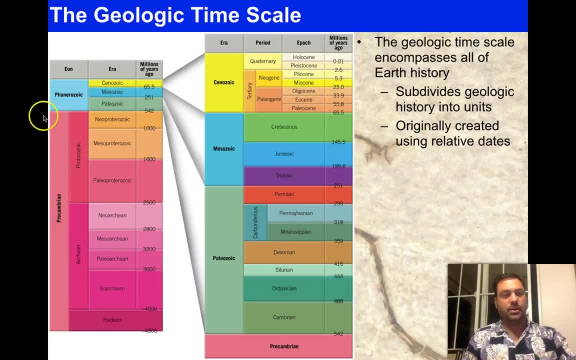 So this is the generalized one. There's a period of time called the Phanerozoic, which is the period of time in which we live, And this is the youngest eon, And below it was a period of time called the Precambrian. 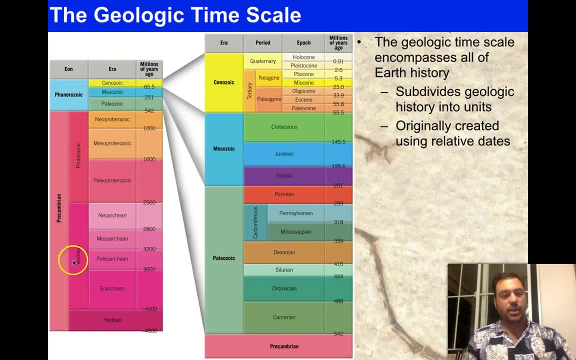 Precambrian is subdivided into the Proterozoic and the Archean, And we'll be talking about that in a future, actually in the next lecture, in detail. What we know most about the history of Earth is in the Phanerozoic. 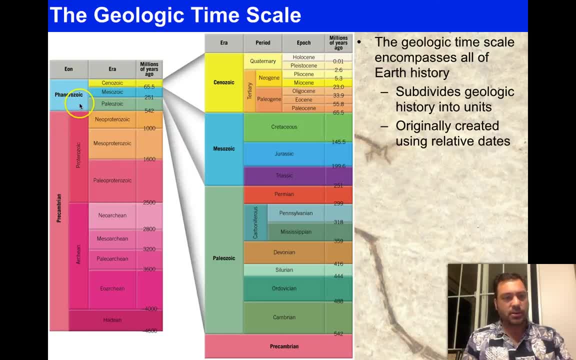 And the reason why is because this is where we have the fossils. right Visible fossils are present in rocks. They're present in rocks during the period of the Phanerozoic, And so we can use fossil succession to figure out everything. 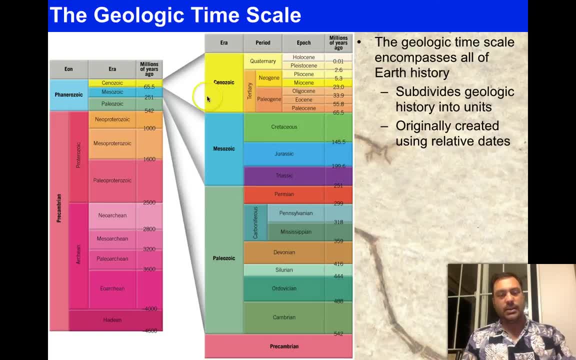 We've got the Paleozoic, the Mesozoic, the Cenozoic, And these can all be subdivided into different groups, The Permian most famous of which is the Jurassic or the Triassic, and the Cretaceous, all right in here in the middle of the Mesozoic. 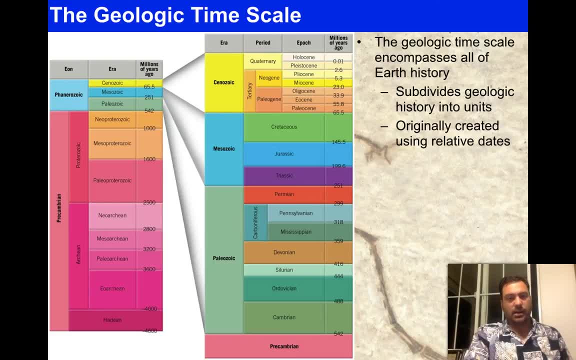 Putting all this stuff together has taken several lifetimes and a lot of hard work, Okay, To be able to put dates to the actual dates. So let's look at the time scale, So the structure of the time scale. we've kind of been going over this really quickly. 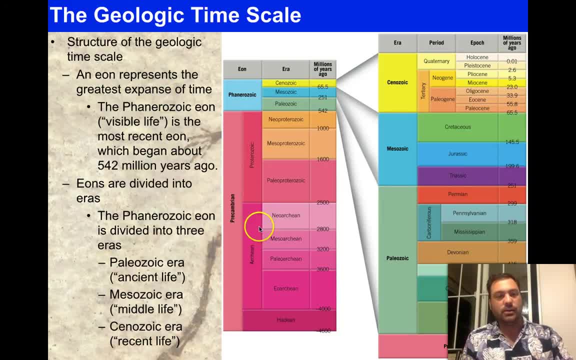 An eon represents the greatest expanse of time. This is an eon. here, The Phanerozoic eon is the most recent eon, which began about 542 million years ago. All right, The Phanerozoic eon has the Paleozoic, which stands for ancient life. 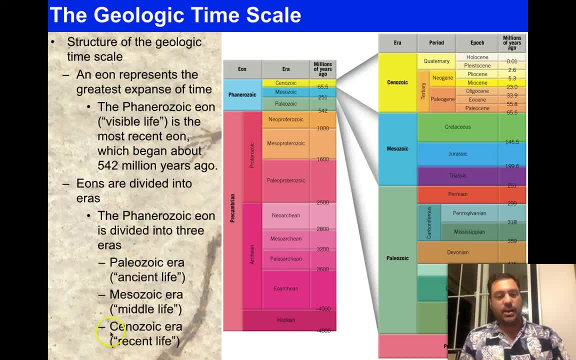 The Mesozoic, which means middle life- This is also known as the age of the dinosaurs- And the Cenozoic era, which is recent life, The age of mammals. So this would be the basically ancient life, middle life or dinosaurs, and Cenozoic is 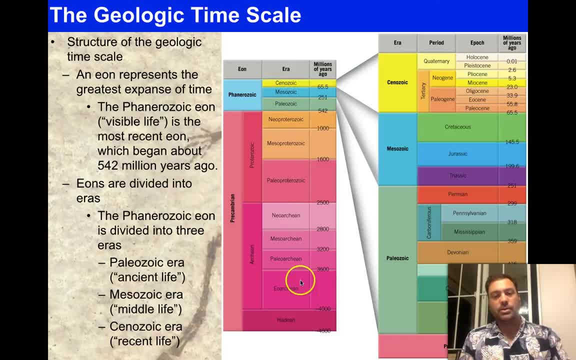 the period of time of the mammals. When you look at all of Earth's history, it's not very long. It's a very, very small period of time right up here at the top, Cenozoic. Now, if we even break up the Cenozoic, we realize that human beings which have dominated the 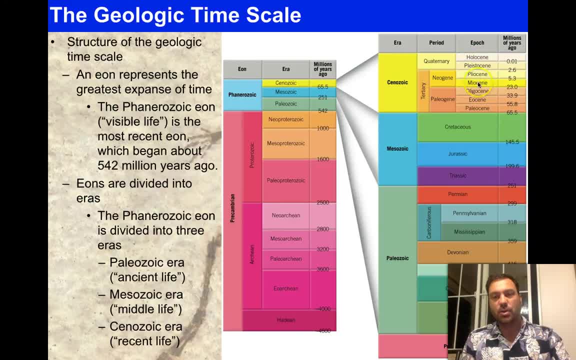 Earth during the period of time of the Holocene is really just a very small sliver of time in the general view of what's going on in the Holocene, The Holocene being only the last 10,000 years, Pleistocene going all the way back 2.6 million years ago. 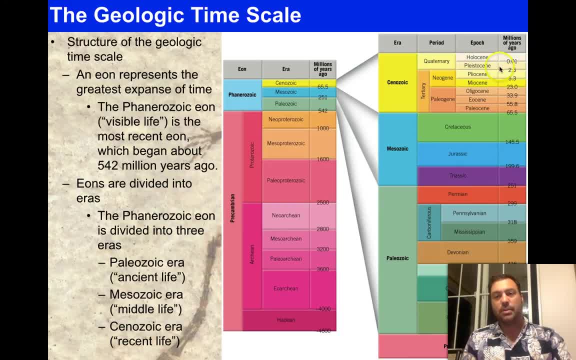 We find evidence of hominids populating the Earth all the way into the Pliocene in Africa. So humans and their origins really are only major players in Earth history in the last 5 million years and really agents of major worldwide change in the last 10,000. 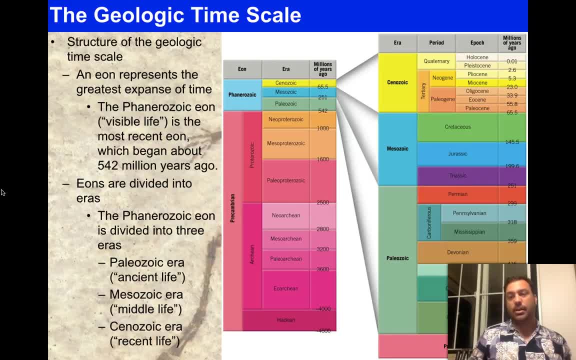 It's extraordinary how much effect we've had During that period of time. During the rest of this we've seen dinosaurs and meteor impacts and all kinds of different things happen. Major extinctions- right Six extinctions that have happened that have almost wiped life out. 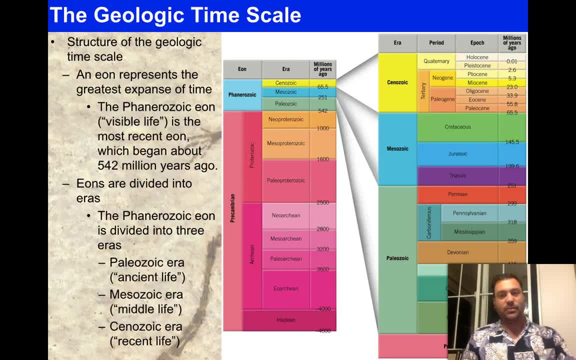 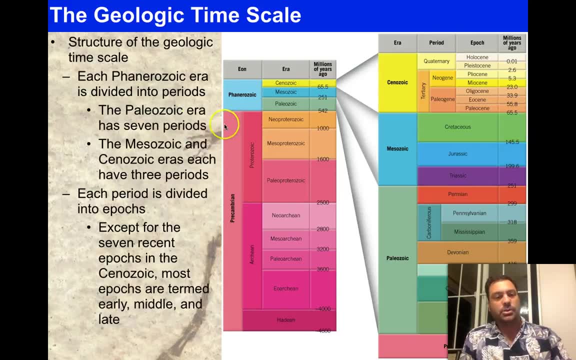 And we're just kind of sitting there right at the very edge up here during the Holocene. So anyways, just some quick notes here. Each Phanerozoic era is divided into periods, So here we see, the Phanerozoic 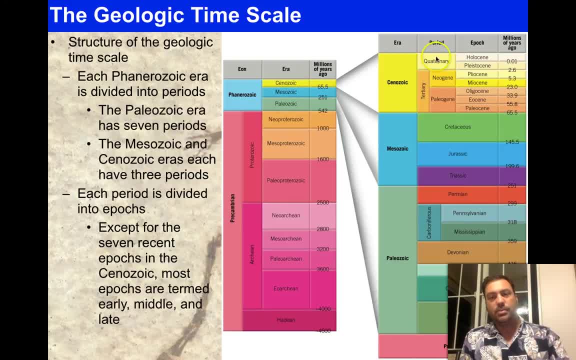 And here are the eras, here And here are the periods, Right, This is what it's talking about. So here we've got the Quaternary and the Tertiary, And the Tertiary in Europe is usually split up into the Neogene and to the Paleogene. 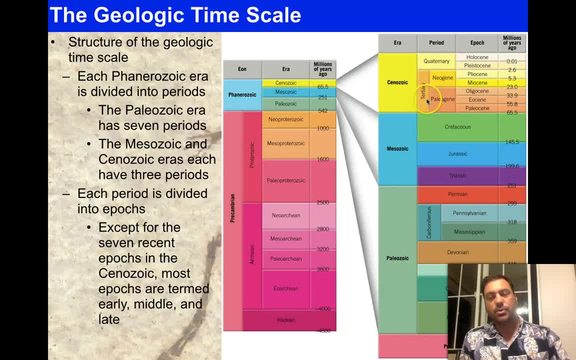 But you get the idea. The Paleozoic era has seven periods, Right Here we see the seven periods here: The Cambrian, the Ordovician, the Silurian, the Devonian, the Carboniferous, if you live. 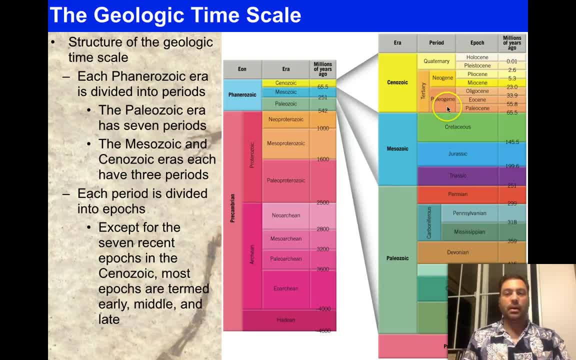 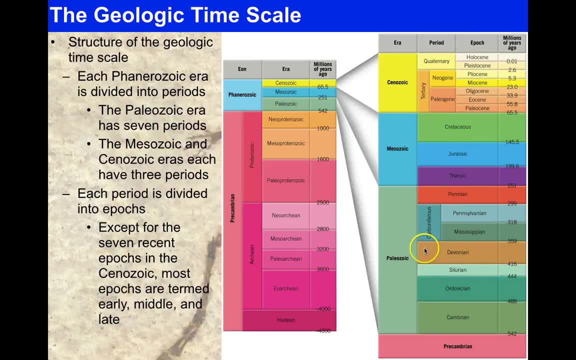 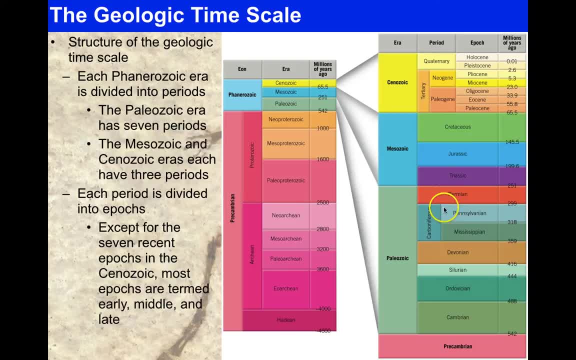 kind of thing. We don't normally do that up here with the Cenozoic And even with the Mesozoic. we usually resist doing that somewhat, But we do that frequently with the Paleozoic. The reason why we do that is we tend to drive the Neogene and the fleeing Neogene into the 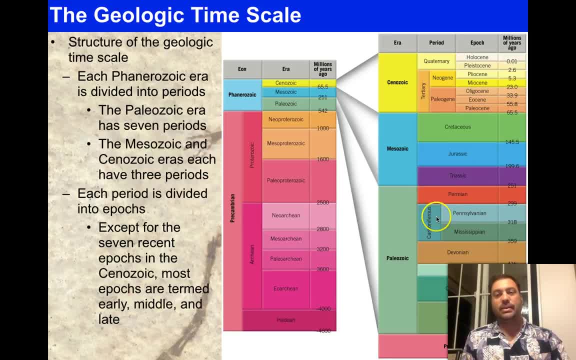 Neogene, And although the Neogene and the Paleozoic are in the Neogene and the Pyrenees, we're not going to do that. Why not? They're not going to be present when the Sun comes out. We're going to keep going. 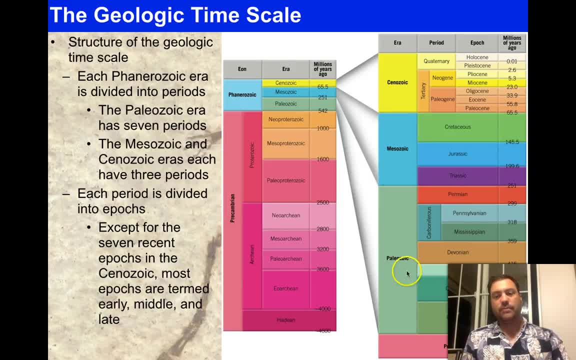 And so you've got the Neogene and the Paleozoic. resist doing that somewhat, But we do that frequently with the Paleozoic, And the reason why we do it is because the periods of time that are here are very, very large. Right, The Permian is lasting a period of roughly 50 million years. The 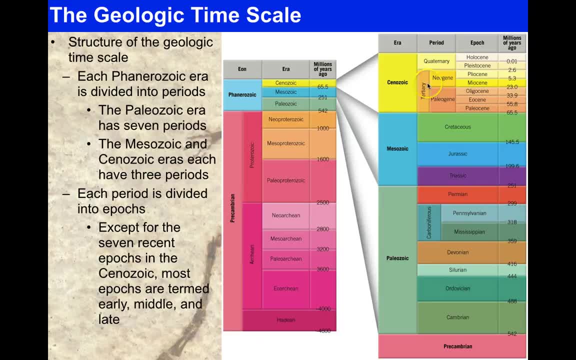 50 million years is as big as the entire Cenozoic. almost Right, Cenozoic means 65 million years, So it's 15 million years longer. The Devonian, of course, is well over the period of time of the Cenozoic. So this is, this is just a huge. 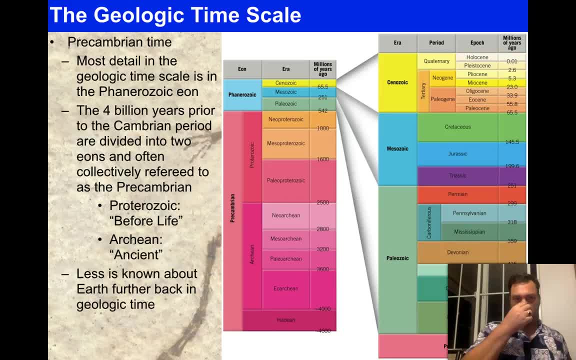 period of time. So most detail in the geologic timescales of the Phanerozoic Era. Right, That's where we have all the fossils. That's what allows us to break it all open. The four billion years prior to the Cambrian period are divided. 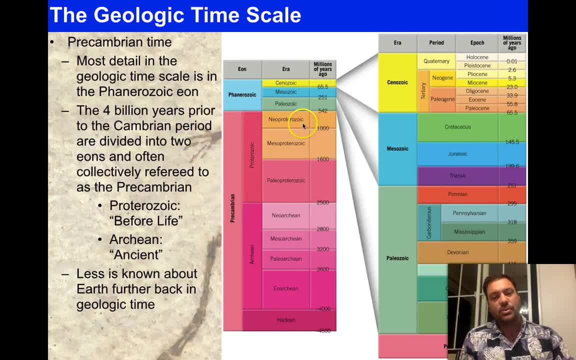 into two eons. This is actually where we know the least history of the Earth. This is a real problem for us as geologists and kind of the keepers and interpreters of Earth history. There's a couple of reasons why, And we'll go into this here momentarily. So it's divided into two eons. 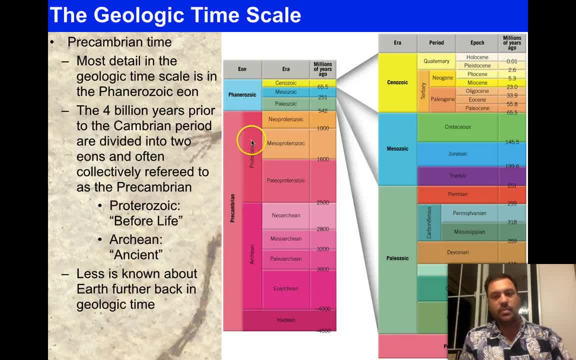 and often collectively referred to as the Pre-Cambrian, everything before the Cambrian. Right. The Cambrian is the beginning of the Paleozoic here. So everything below the Cambrian is the Pre-Cambrian. That's what this all is, Okay. 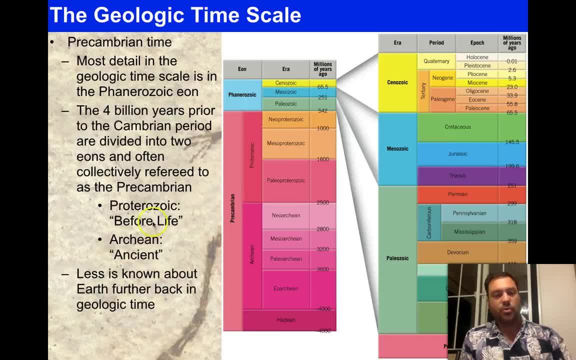 And during these period of times, during the Protozoic, which means before life. it was called that because all of a sudden, when you get into the Paleozoic, we start seeing fossils, we start finding shells and teeth, But before that we find 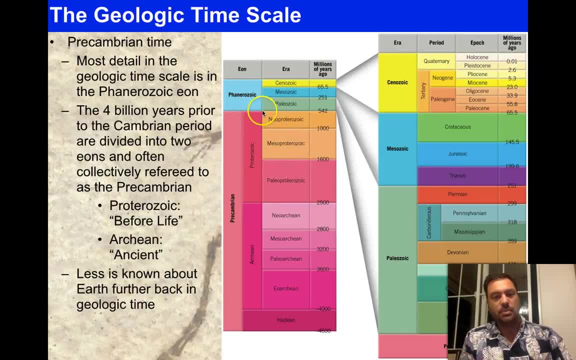 nothing, right Almost nothing, And so people believed that there was nothing here. Now they know that in fact, there had been life all throughout this period of time. It just took us a long time to find those fossils because they didn't have the hard parts right. They didn't. 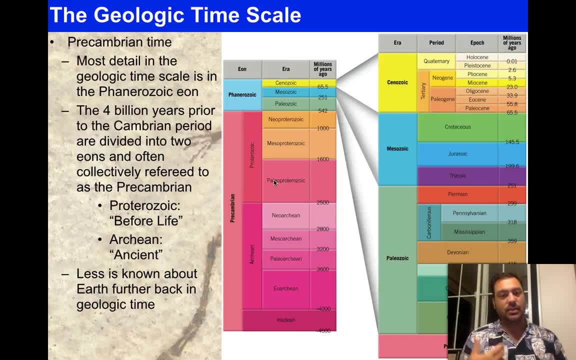 have the fossil or the bones and the teeth and whatever it is that we now find in most of our phanerozoic fossils up here. These things were all soft-bodied And, of course, the Archean is the period of ancient time, The Neo-Archean, the Meso-Archean, the Paleo-Archean and the Eo-Archean. 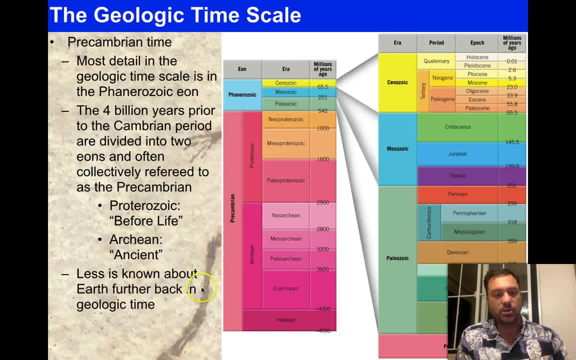 all part of the Archean period of time, Very, very ancient, And less is known about Earth further back in geologic time. Why? Because plate tectonic processes in the rock cycle destroy old evidence. If there was any fossils there, most of them are destroyed. We get lucky from. 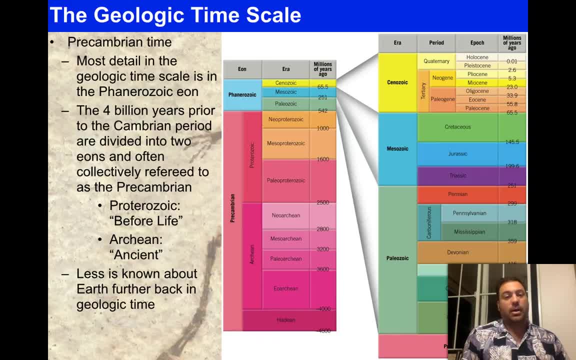 time to time We find some evidence that for the most part you know you have plates run into each other, You get metamorphism, and the metamorphism destroys the evidence of any life, And so it's very difficult to date these things and put together these. 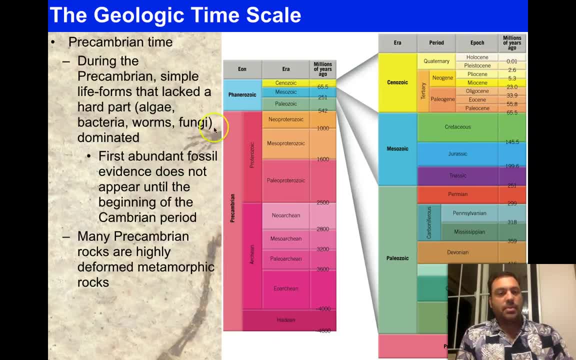 stories. So it was during the Precambrian simple life forms that lacked a hard part: algae, bacteria, worms, fungi dominated. You know, the first abundant fossil evidence does not appear until the beginning of the Cambrian- We just talked about that- And many Precambrian rocks. 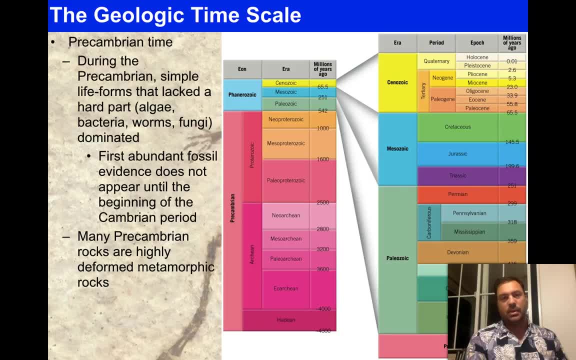 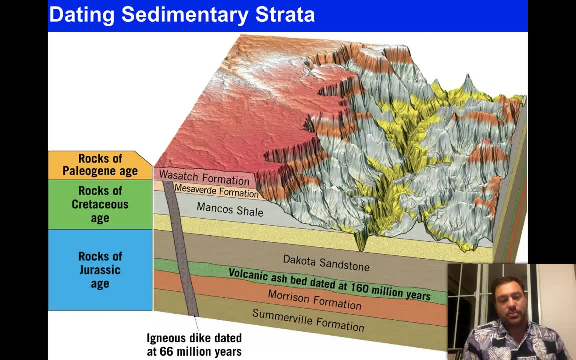 are highly deformed metamorphic rocks. There's just nothing to find in them, So the evidence is very scant. But that doesn't mean that we can't put some of the evidence that we have in the research to work on. It's really important that we have these principles to work to be able to 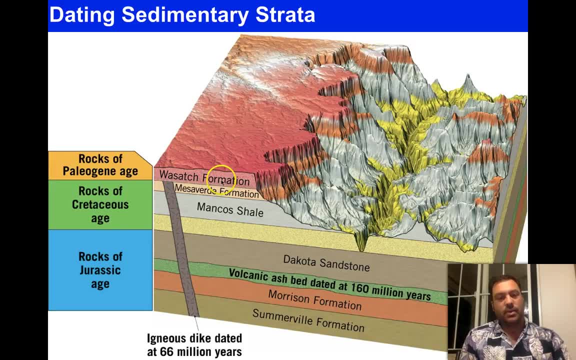 figure out some of these problems. So, for example, here we see a canyon, The top of it of which is the Wasatch formation. Down below is the Somerville formation. We have a bunch of rocks in sequence in between. We can put together a really cool kind of sequence of events that have happened here. 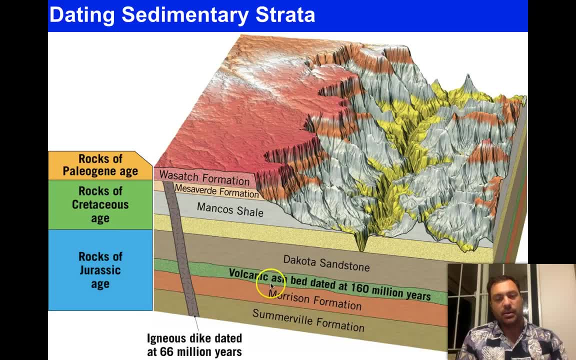 because we know that we have minerals, a volcanic ash bed that's going to have potassium argon in it, And we can go through and we can date that, And in this case they've said: oh, it's 160 million years old. 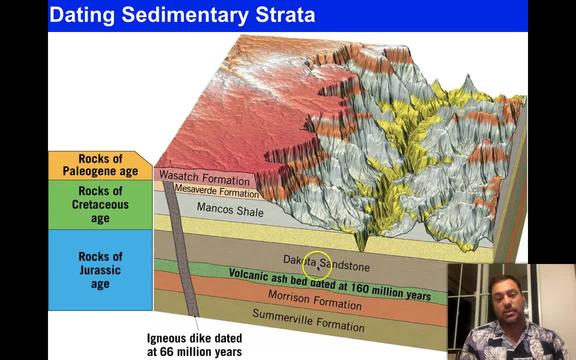 And we know that it's. that means everything above it is younger than 160 million, Everything below it is older than 160 million years old. And then we find an igneous dike that is intruded here, but it doesn't intrude the Wasatch formation, right. 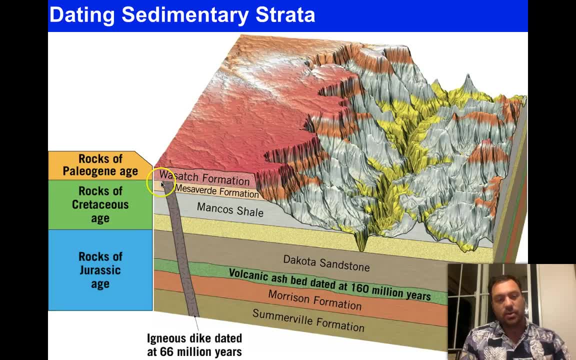 It's clearly younger than Wasatch because it doesn't cut across it And that's at 66 million years old. So the Wasatch formation has to be of the Paleogene age, because the Paleogene started 66 million years old. Okay. 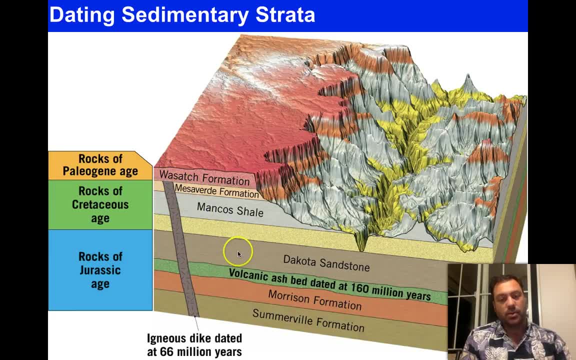 The Mesa Verde formation, the Mancos, the Dakota, all of these things. we know what these, where these should fit in. These should be of Cretaceous age, The Jurassic age rocks, the Morrison, the Somerville. we know where those are as well. 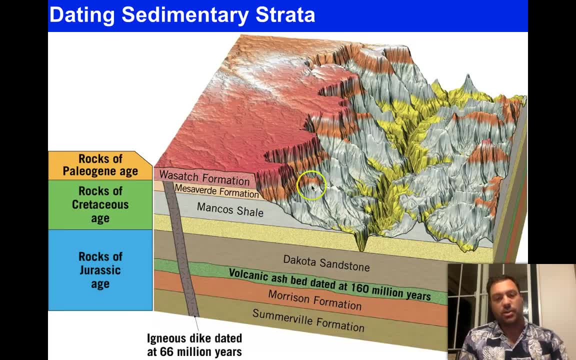 Okay, You get the idea. And so the Mesa Verde formation. we can assume that these also exist over here. Why? Because we can assume original horizontality and that these things were continual. right, There was continuity between or across these units here. 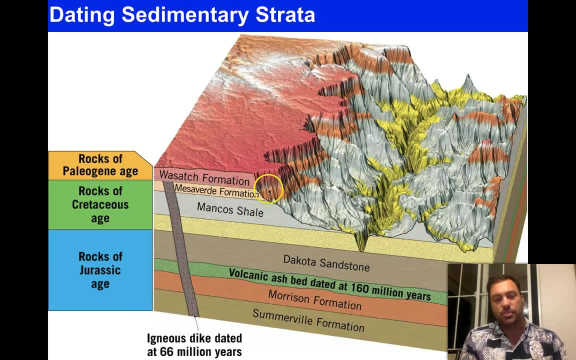 We see continuity here, We can assume continuity here, And we can assume continuity here here, and then, as well as that, pink over to the Wasatch as well, So we're able to put together a whole process that since the uplift of the Wasatch we've had the erosion and deep incision by some type of river system into the valley.